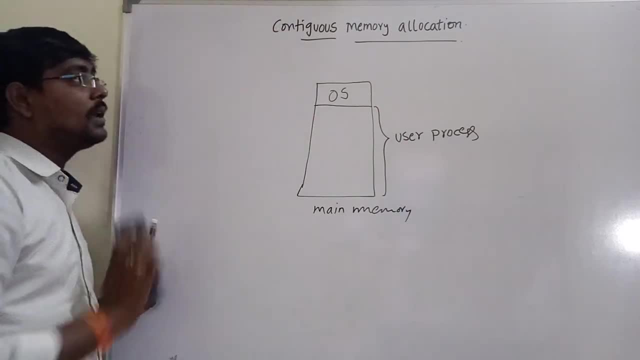 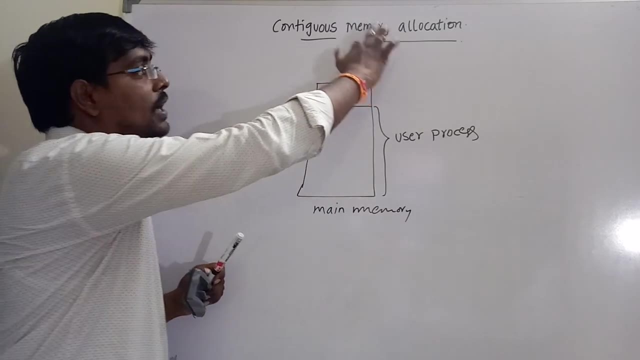 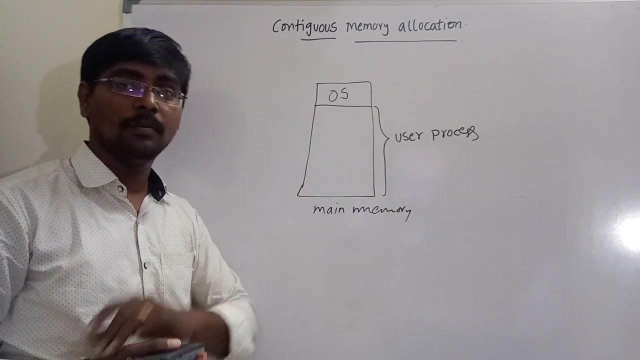 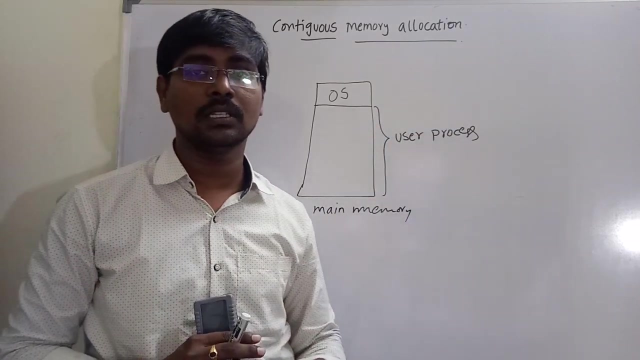 After that contiguous memory allocation is done. Contiguous means: the name specifies. Contiguous means sequential- Sequentially we are allocating the memory. Suppose if a process comes, That process brings one section of the memory That is contiguous to the next process. That is all the process. The memory is allocated sequentially. 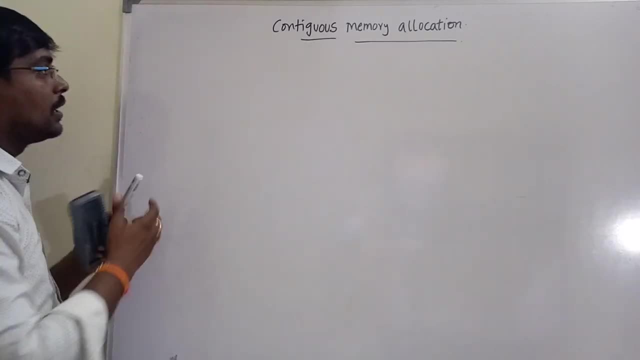 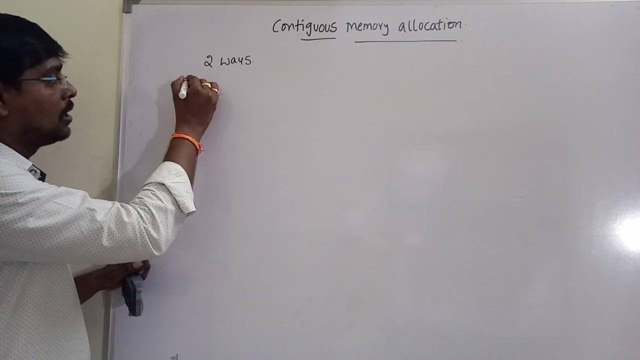 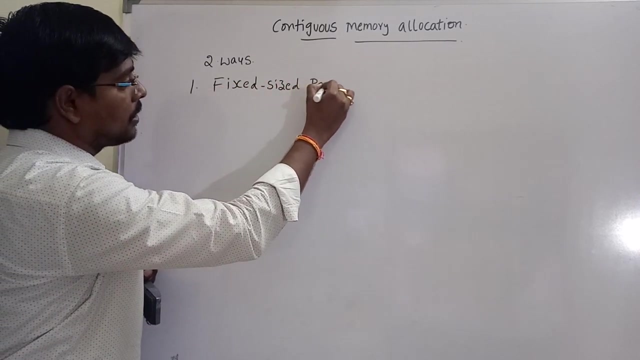 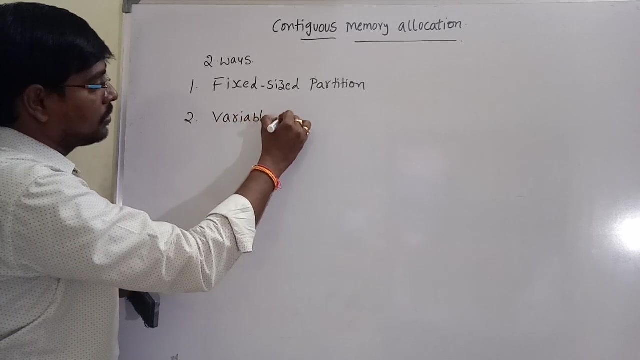 Now we will discuss. Now we will discuss In memory allocation We have. We have two ways. We have two ways of memory allocation. First one is fixed sized partition. Second, one variable sized partition. Second one is variable partition. In these two ways we are allocating memory. 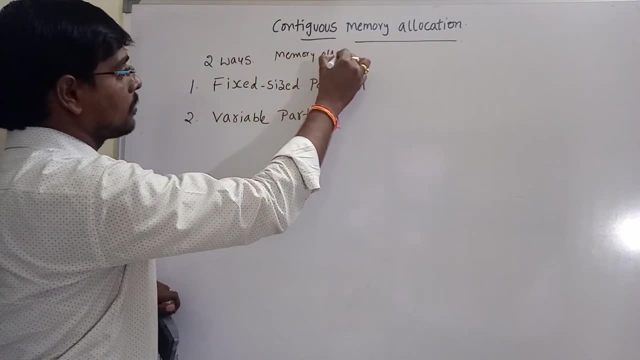 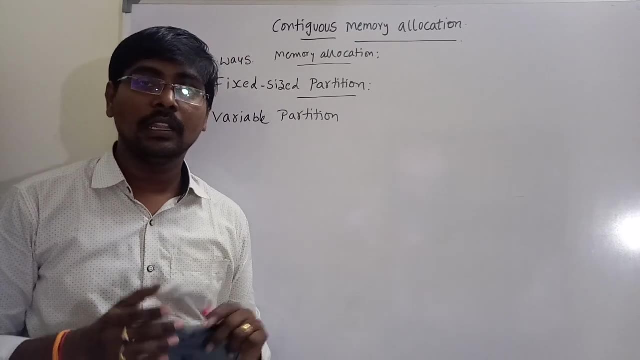 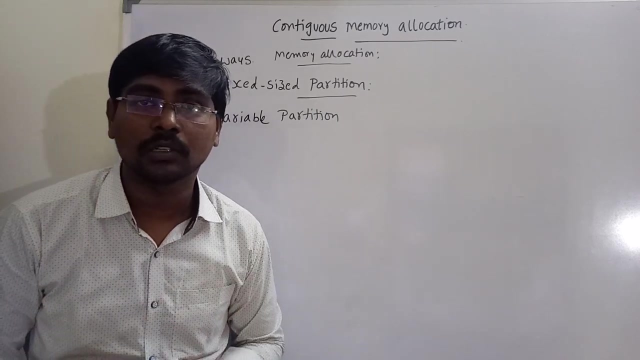 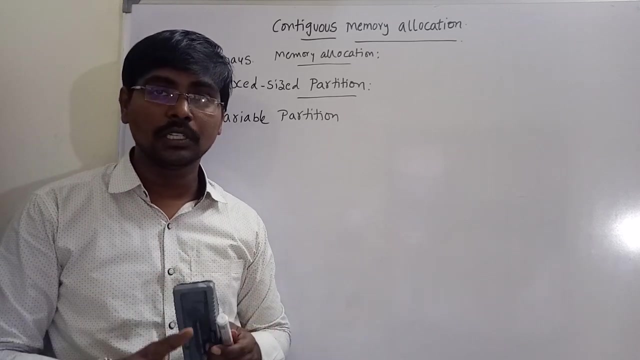 This is memory allocation. So first move to fixed sized partition. Here the total available memory Ignore operating system memory. We are concentrating only on user process memory. Here the total available memory is divided into partitions of fixed size. Fixed size means the size of each partition is same. 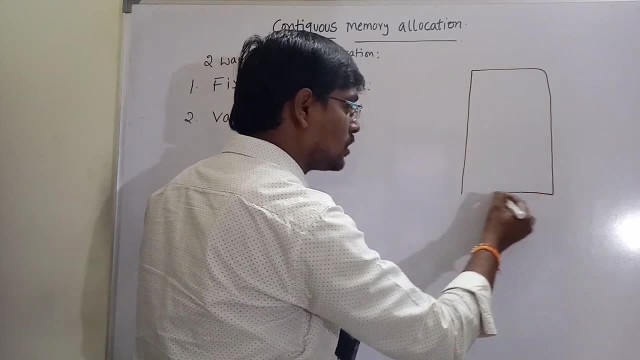 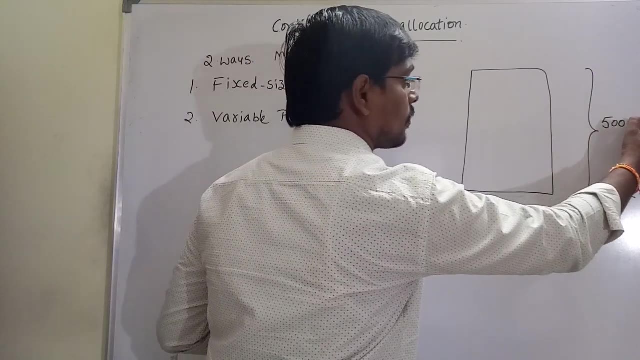 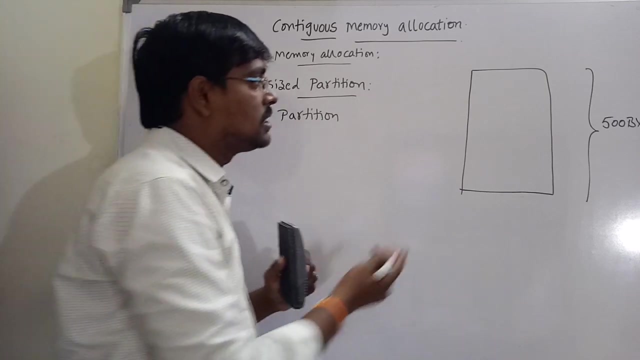 For example, this is the memory, This is the user process memory. For example, assume the size of this memory is some 500 MB, 500 bytes. Assume the size of this memory is some 500 bytes. Now my memory is divided into fixed partitions. 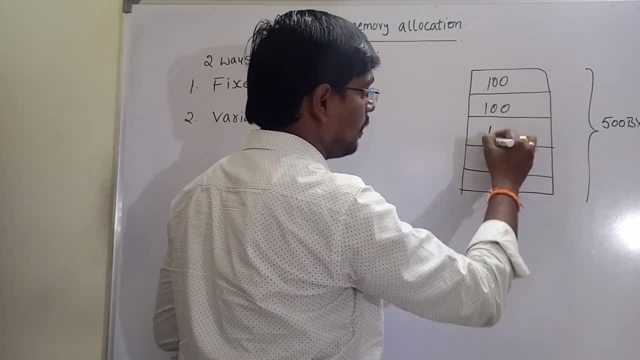 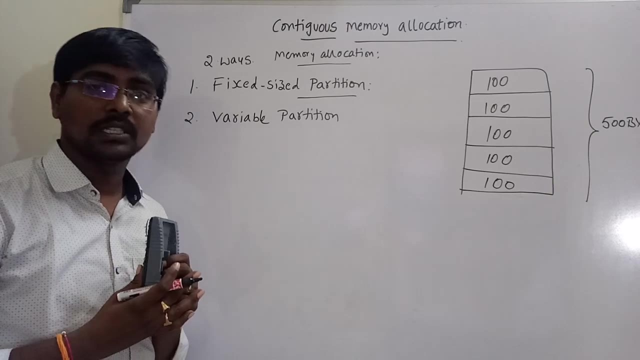 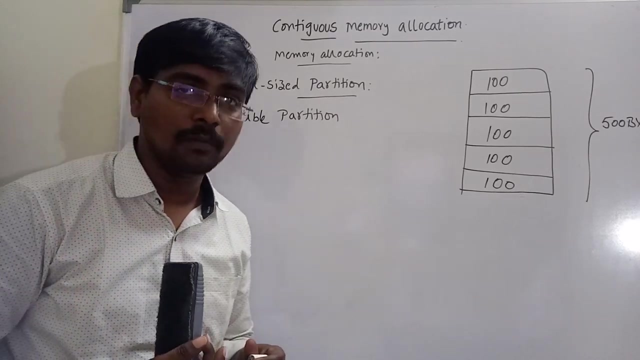 That is the size of this one is 100.. 100.. This is the way I am dividing my memory. Whenever a process comes, What we will do. Whenever process enters into the system, That process is placed into the input queue. A process is placed into the input queue. 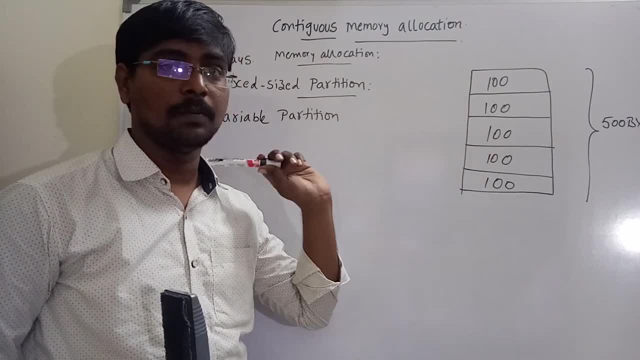 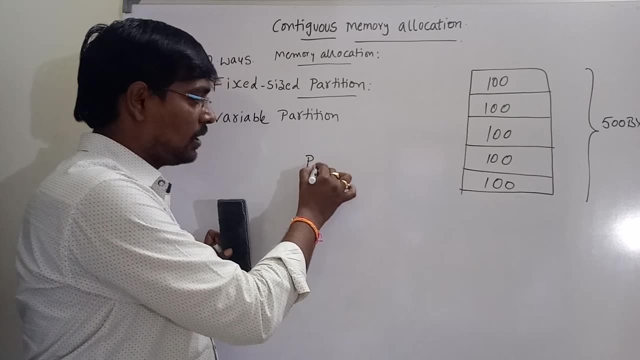 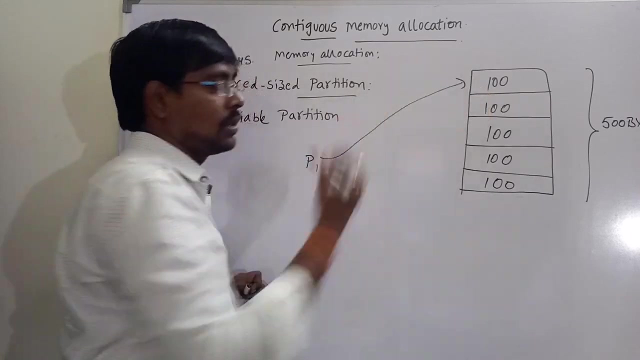 First, whenever a process request for the CPU For that process we are allocating one partition, For example process P1, enters into the system, It requires some memory. What we will do? Assign this partition. Suppose the process P2 enters into the system. 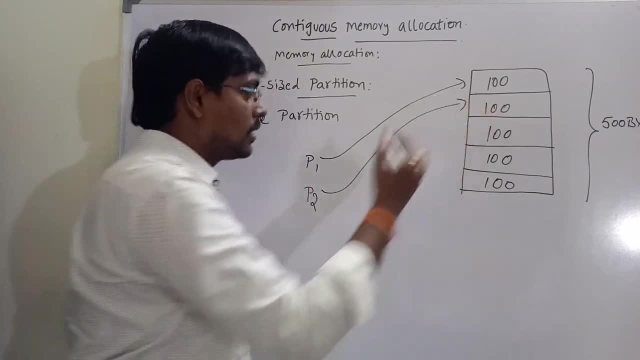 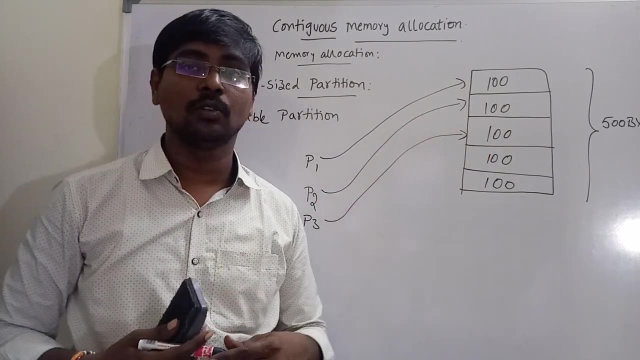 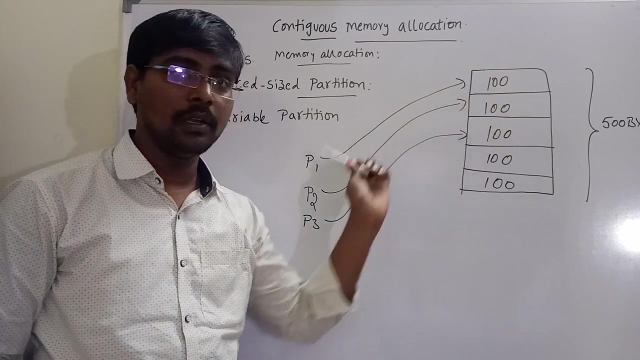 It requires some memory. In the similar way, suppose the process P3.. Whenever a process enters into the system, We are allocating one block of memory to that particular process. One block of memory to that particular process, For example, if process size is. 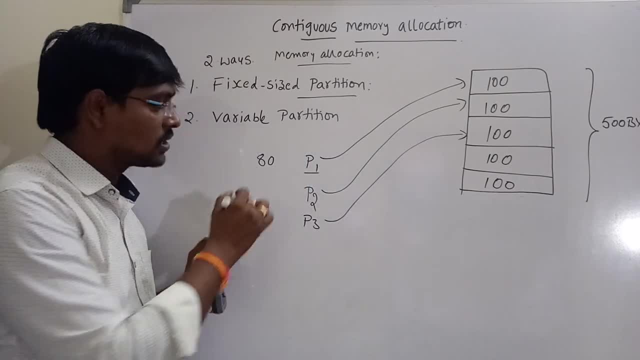 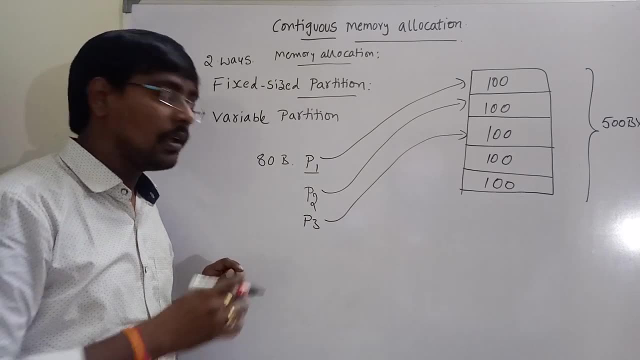 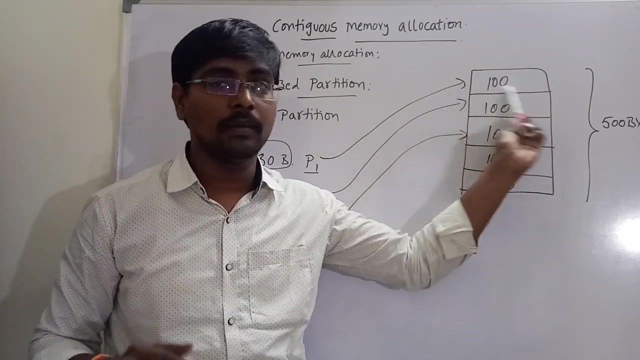 Process size is some 80.. Process size is only some 80 bytes, But the partition size is 100 bytes. What we will do, Even though the size is smaller than the available size, We are allocating complete 100 bytes to the process. 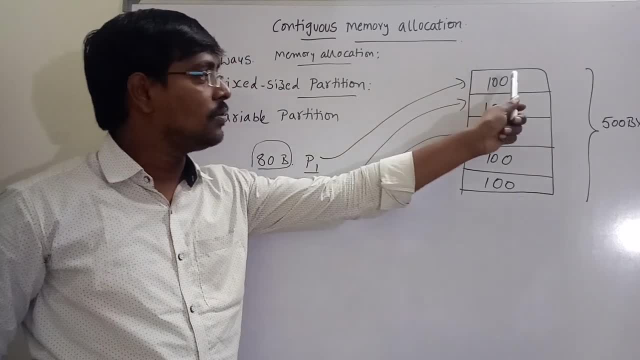 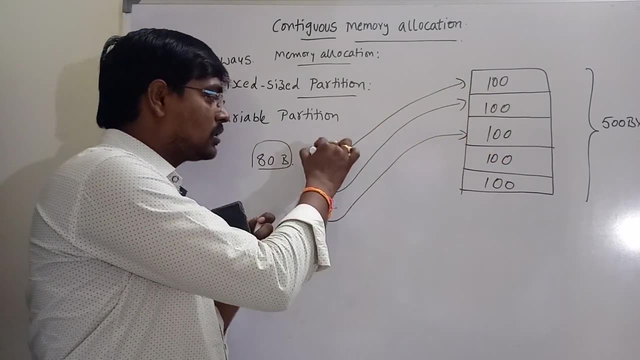 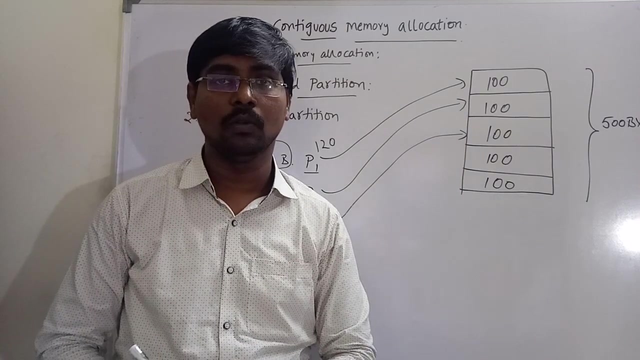 To that the point: Whatever the size, We are definitely allocating 100 bytes of memory to that particular process. For example, if process size is some 120. What will happen For this process? we have no memory is available For this process. no memory is allocated. 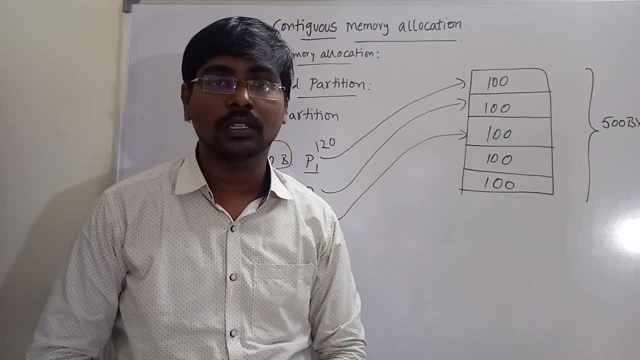 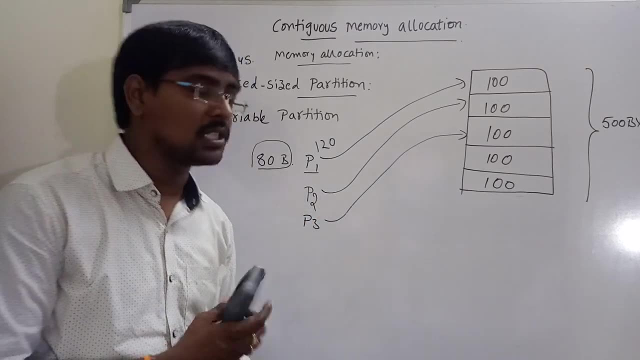 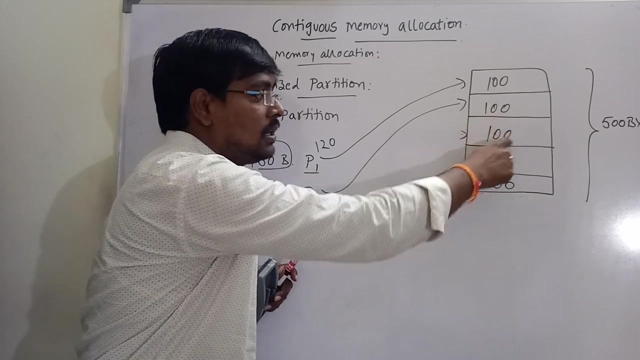 This is the way we are assigning memory to the process. Whenever a process terminates, What happens Whenever a process terminates, That is, completes its execution, Completes its execution, This memory is makes available. This is the memory. This is the free memory. 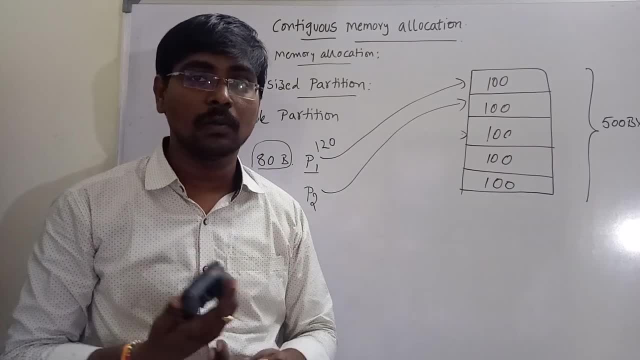 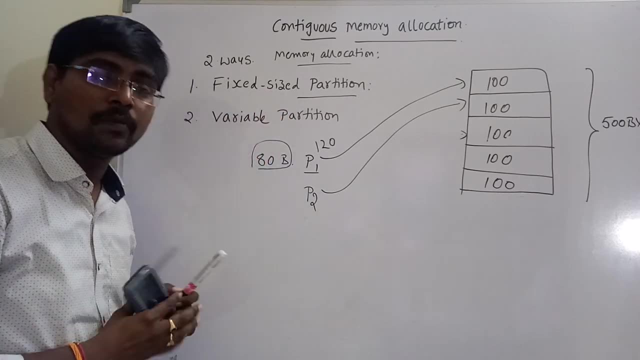 This memory is makes available for the next process. Available for the next process. This is the fixed size partition Here. how many number of process at a time runs Simply depends on the number of partitions. For example, this contains 5 partitions. 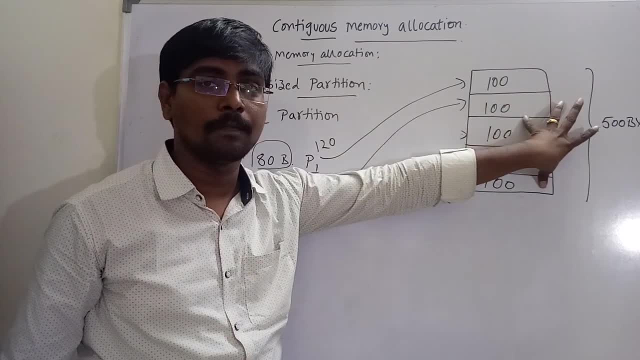 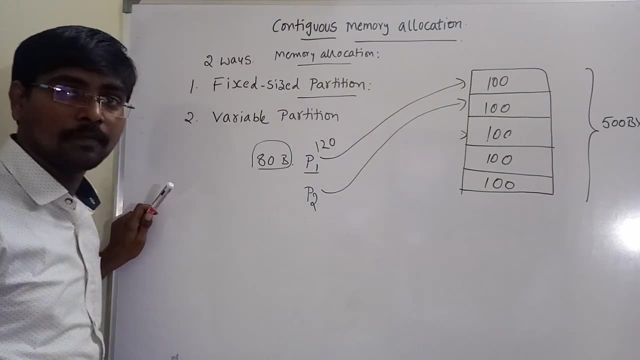 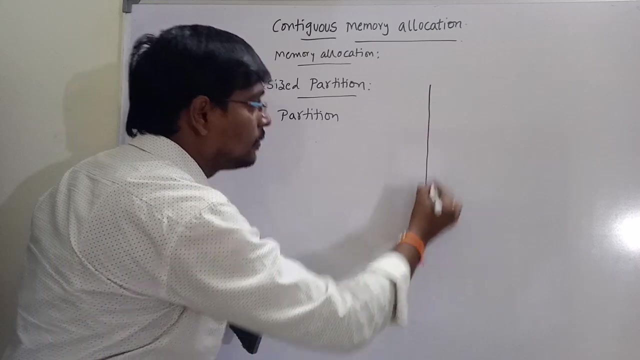 We are allocating a maximum of 5 process at a time. We are allocating a maximum of 5 process. Now come to variable partition. Now come to variable partition Here. what is the concept? This is the main memory. This is the main memory. 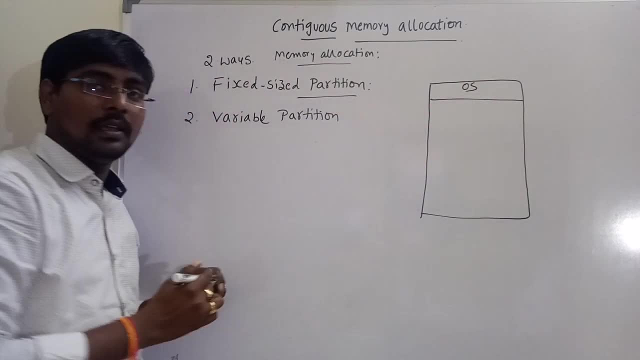 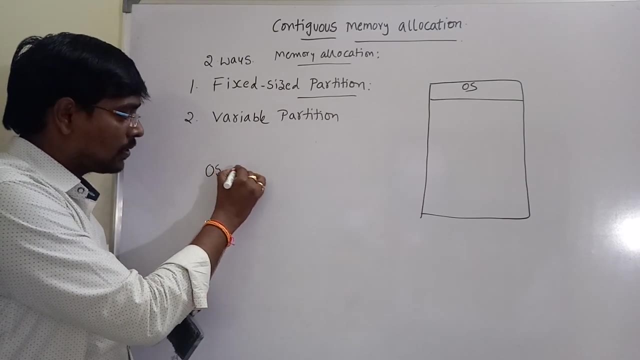 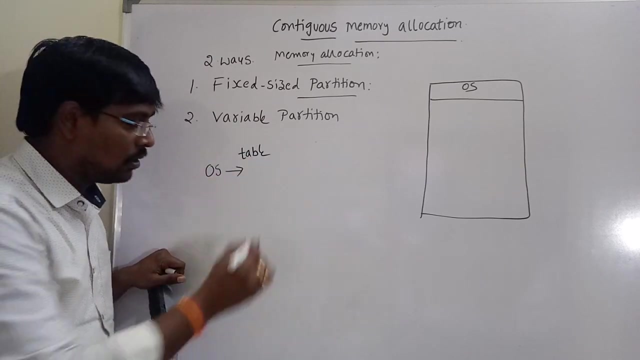 Suppose this is the OS, This memory is allocated to different process. How, In this operating system, In variable partition operating system, maintains a table. Maintains a table. It consists of two parts. It consists of two parts. What are the parts? 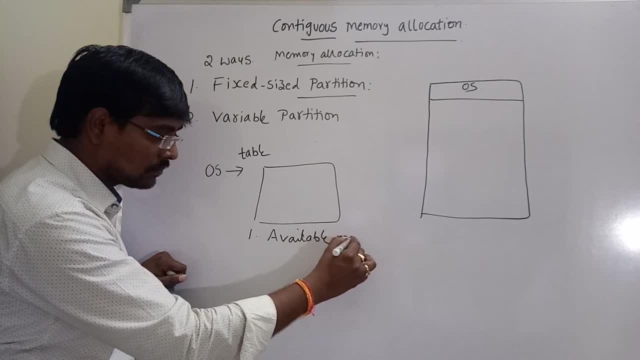 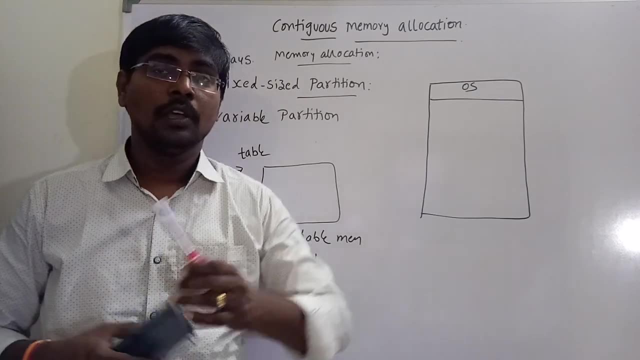 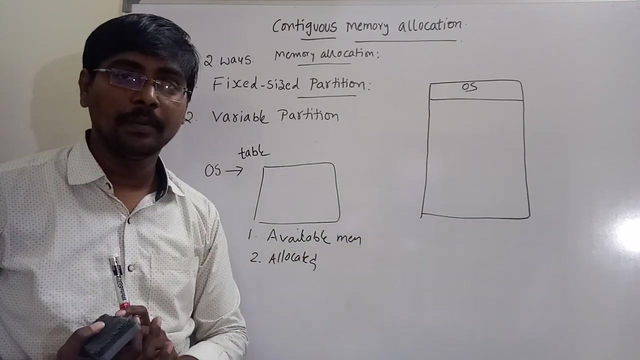 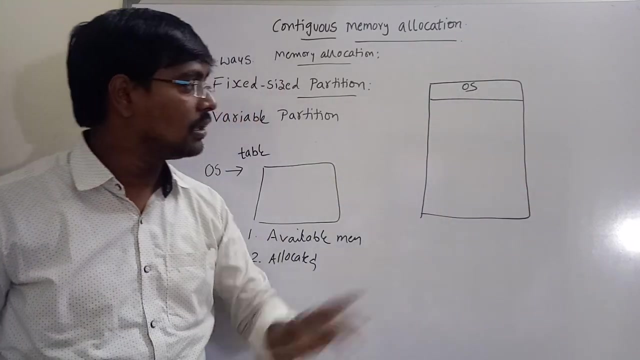 Available memory and allocated memory. So operating system maintains a table which contains the index of available memory and allocated memory. Suppose, if you are not understanding this one, ignore. This is the complete memory available Initially. this is the complete memory available for a process. 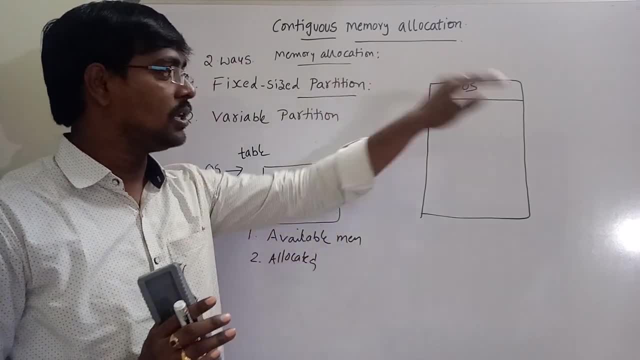 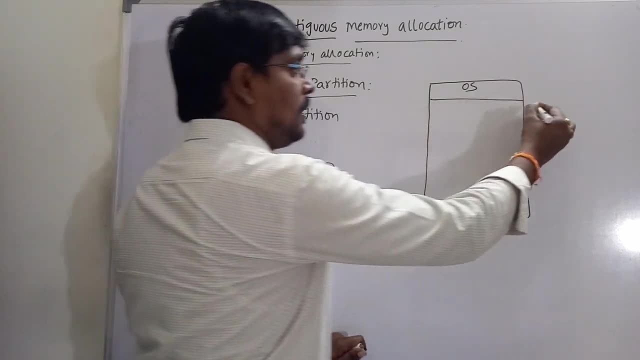 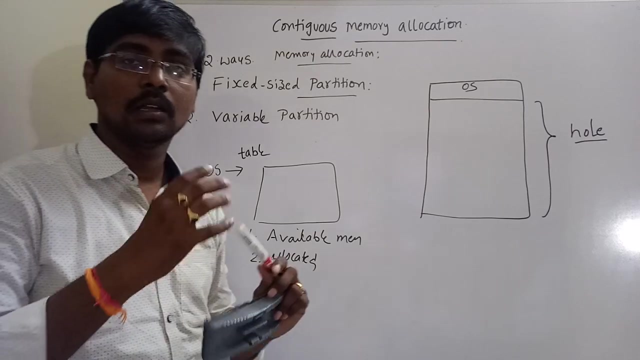 Here no partition is done. In fixed sized partition initially we have divided memory into different blocks. But in variable partition no partition is done. This complete available memory, initially called as whole- The meaning of whole means the large available free memory- is called whole. 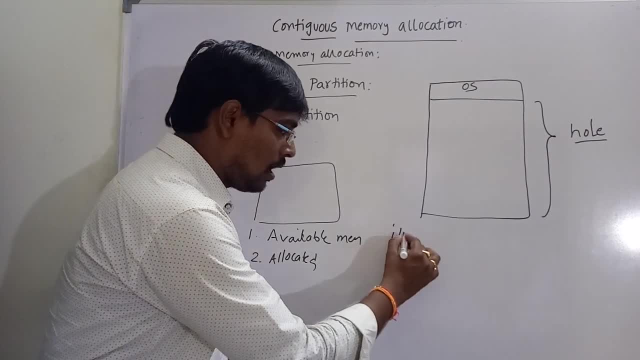 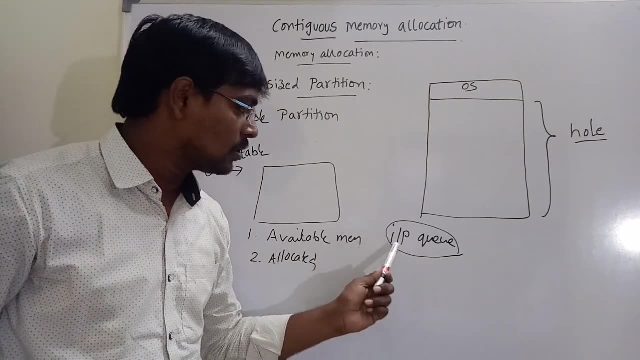 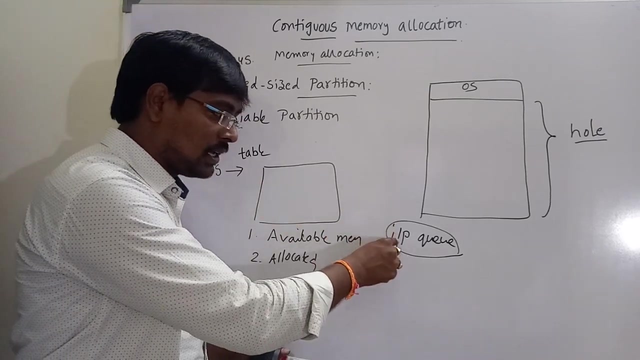 Whenever a process enters into the system, all the process are placed in input queue By default. process enters into the system, The processes are placed into input queue First. operating system selects a process from the input queue. Select a process from the input queue. 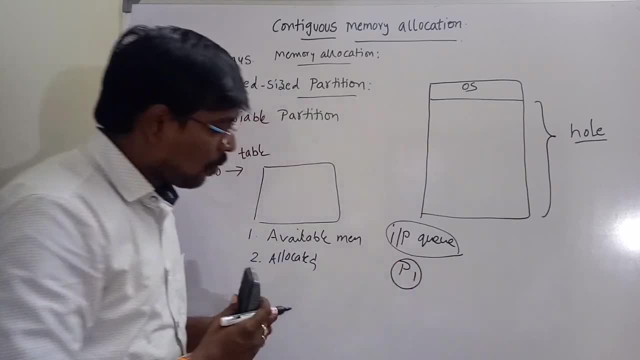 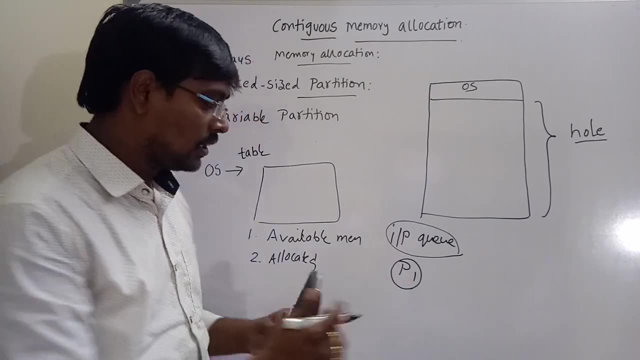 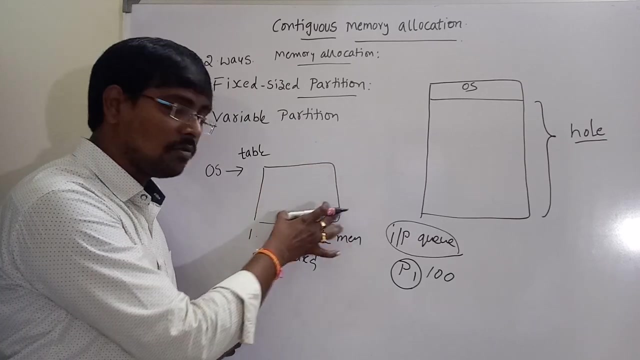 For example, process P1 is selected, What is the memory requirement for this process? Check the memory requirement for this process. For example, this process requires 100 bytes of memory. It checks the table whether 100 bytes of memory is available or not. 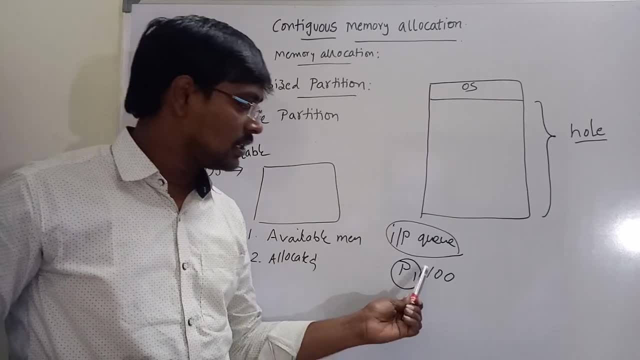 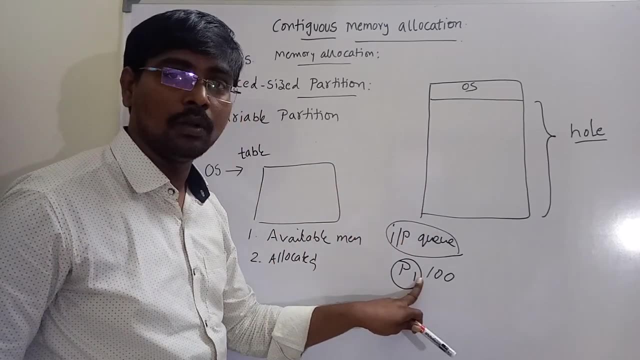 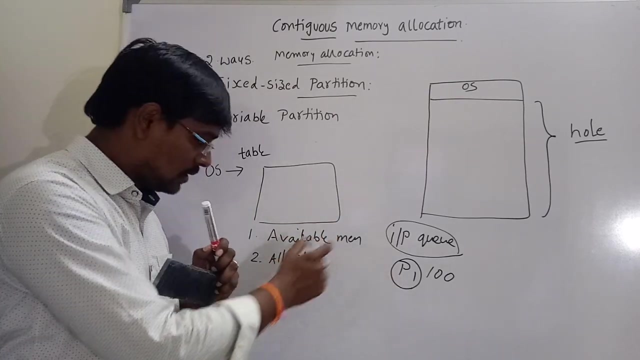 So you got the question First. it picks a process and check whether the requirement memory is available or not. If the required memory is available, we are allocating that process. We are allocating this process and update the table. Update the table means the 100 bytes of memory available. 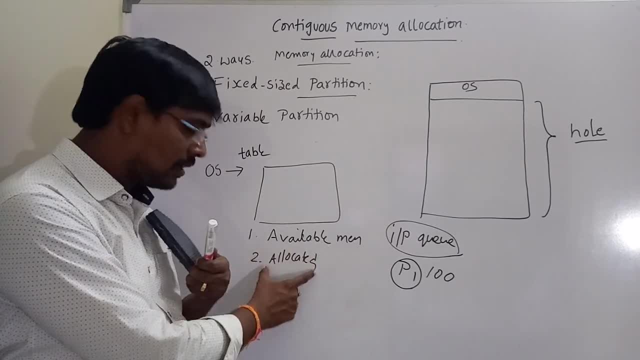 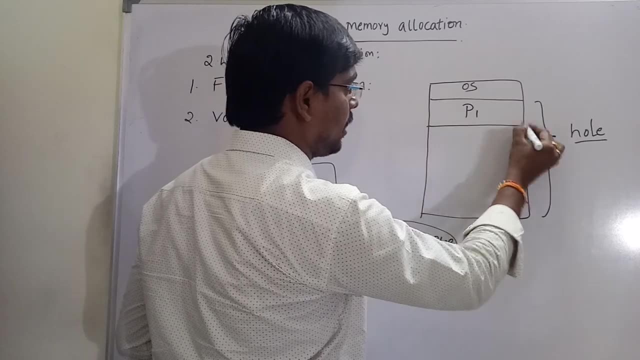 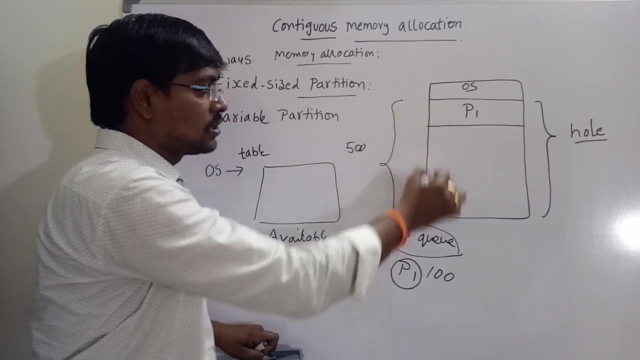 The number of bytes of memory available is decreased and it is added to allocated. So for example, first process P1 enters into the system, It occupies 100 bytes of memory. Assume initially, we are assuming total 500 bytes. Suppose this user space, again 500 bytes. 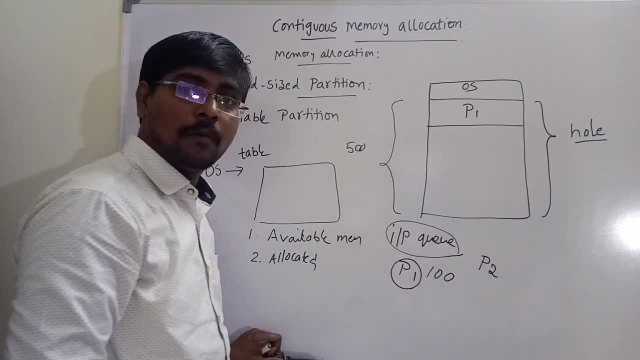 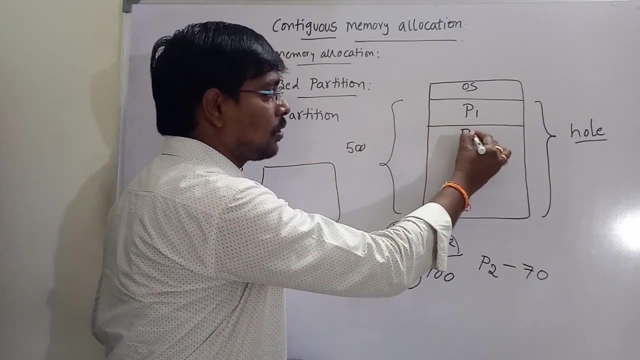 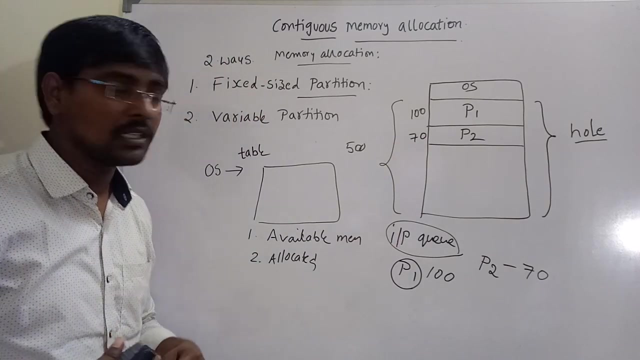 Next process P2 enters into the system. For example, process P2 requires only some 70.. We are allocating process P2.. How much amount? This is 100.. This is 70, only Compare to previous one. In the previous one, first process, 100. 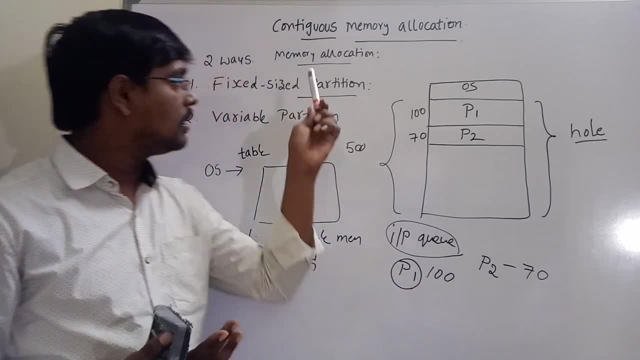 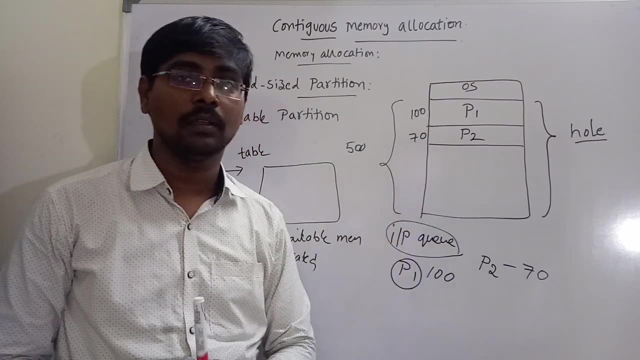 Second process: 70.. Total 170.. But in this method we are allocating 200.. But in this method we are allocating only 100 plus 70 variable, For example, next to process P3, it requires some 200. 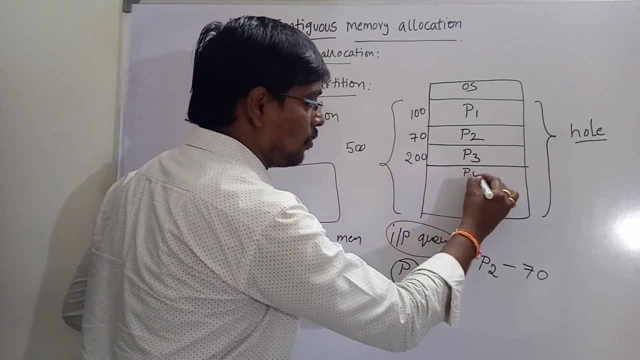 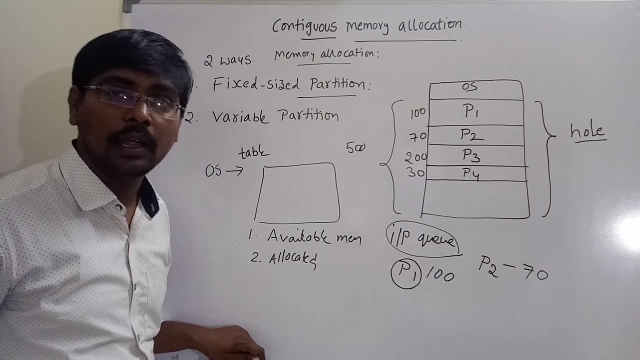 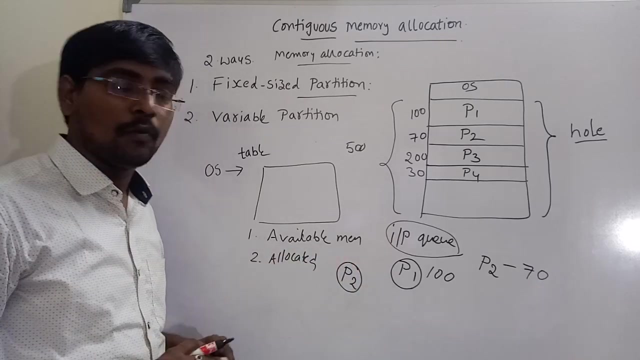 I am assigning 200.. Next to process P4, suppose requirement of process P4 is 30. So how much completed? 300, 400.. Only 100 bytes of memory is available. Assume if process P2 is deleted. whenever a process is deleted here, it forms a hole. 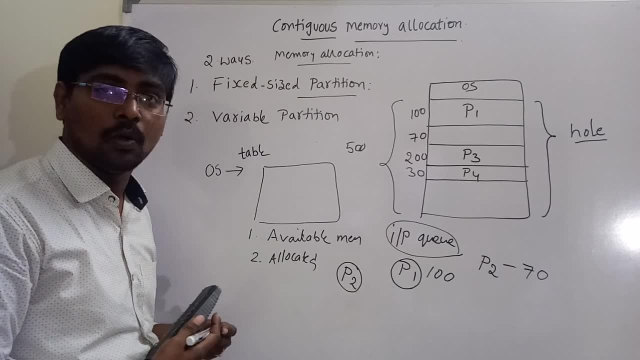 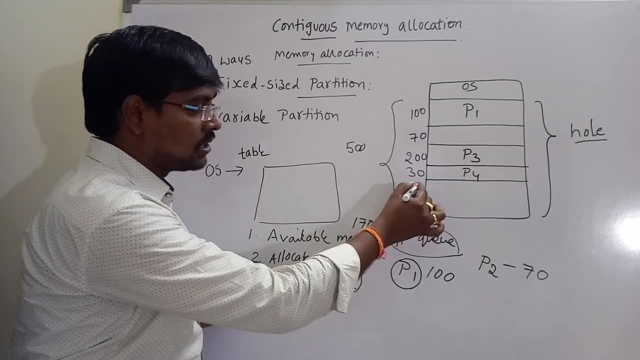 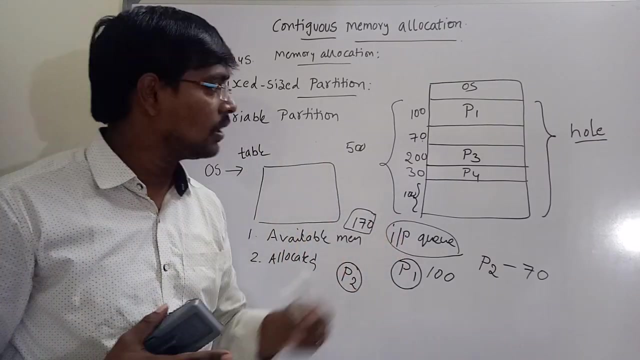 Whenever a process is deleted, it forms a hole. How much available memory Now? available memory is 170.. This space is 100.. That space is 70.. Total available memory is 170.. Whenever a process enters into the system, it checks the memory. 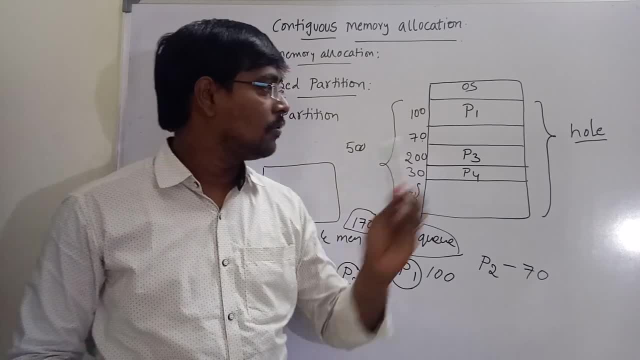 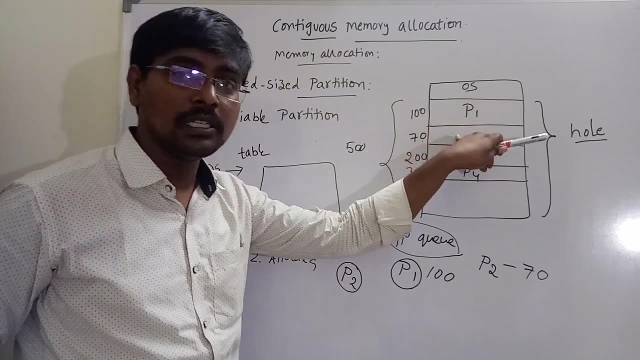 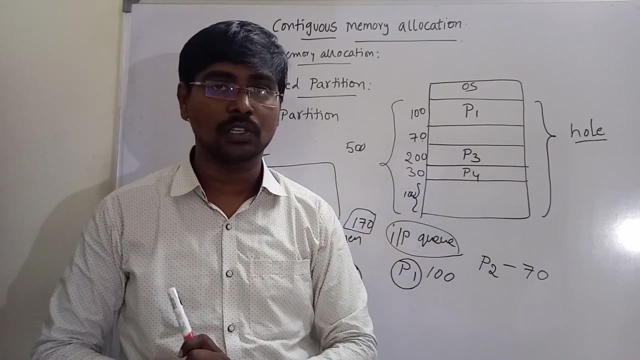 Whether it is available, allocate the memory. Whether it is not available, simply wait in the input queue. Whenever a process terminates, its memory is freed, That is, it is added to available memory. Here we have some problem of fragmentation. At the end of this topic we will discuss fragmentation. 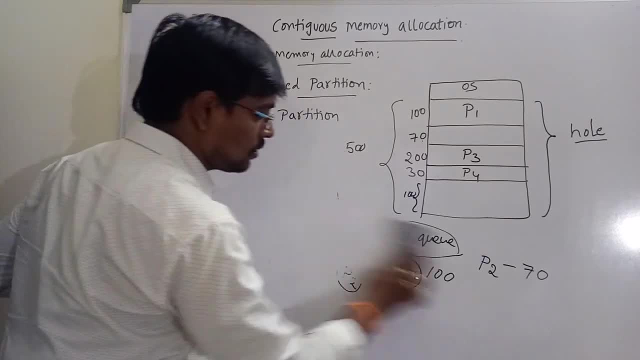 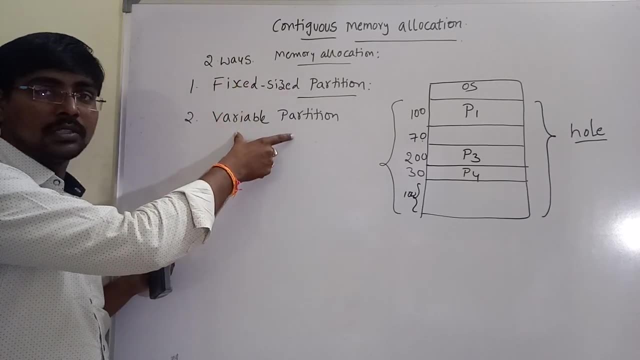 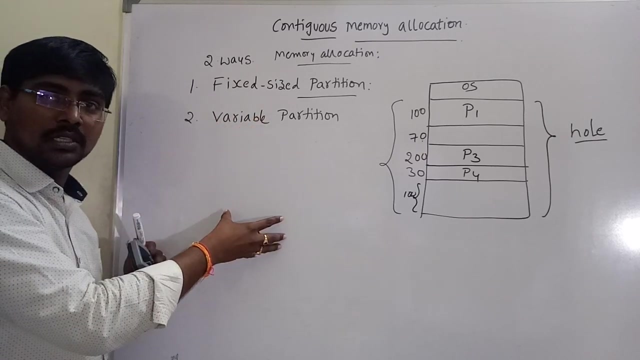 Similar same diagram is placed here. So this is the variable size partition. You got the clear idea of fixed size and variable size. Fixed size means we divide into partitions of fixed size. Variable means, whenever a process comes, add into the free available space. 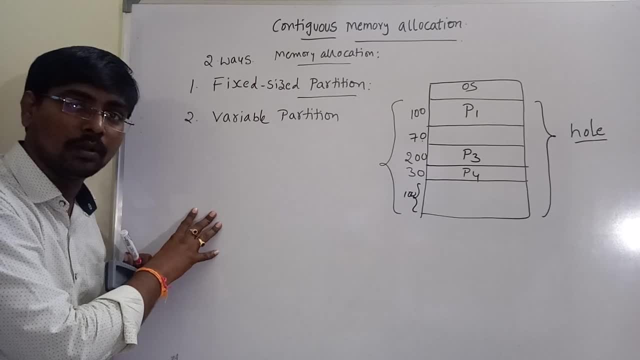 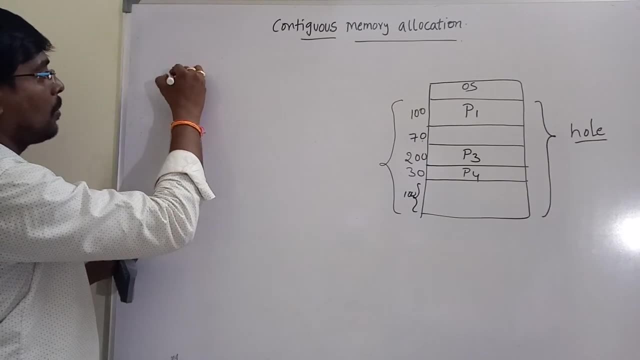 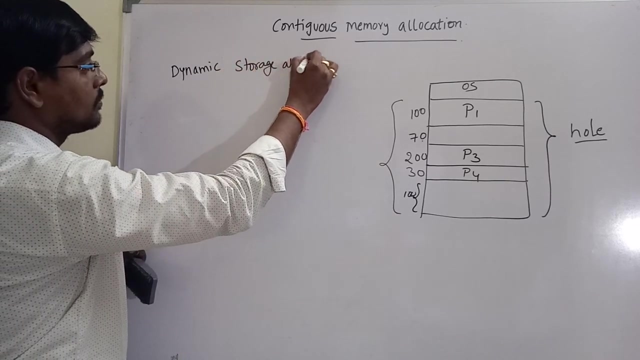 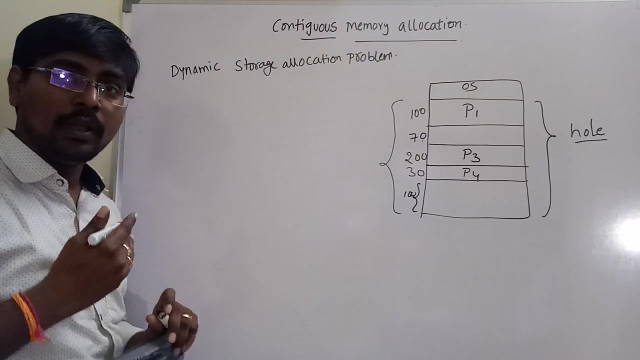 Whenever it terminates, add to the operating system Operating system table. In this memory allocation we are getting a problem. The problem is dynamic storage allocation. Dynamic storage allocation problem occurs. What is the problem? How we are dynamically allocates a process to the memory. 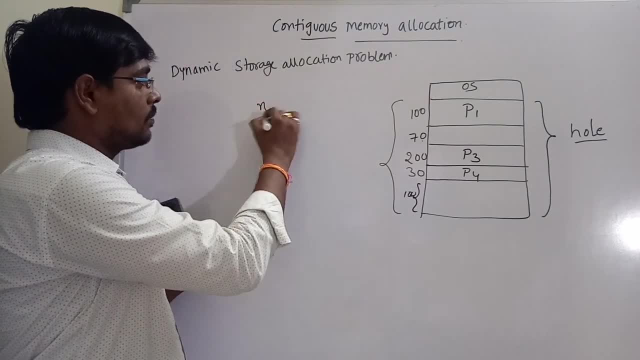 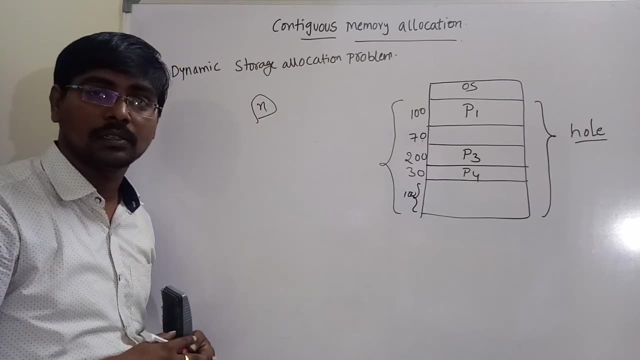 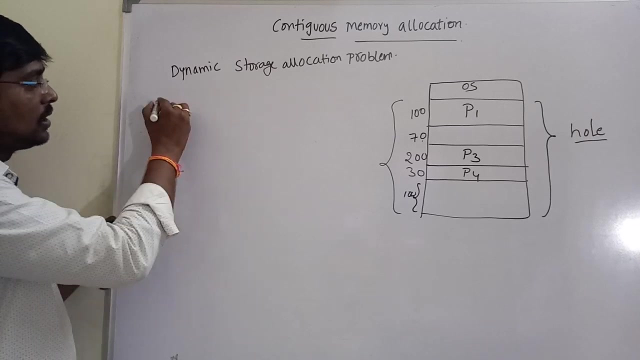 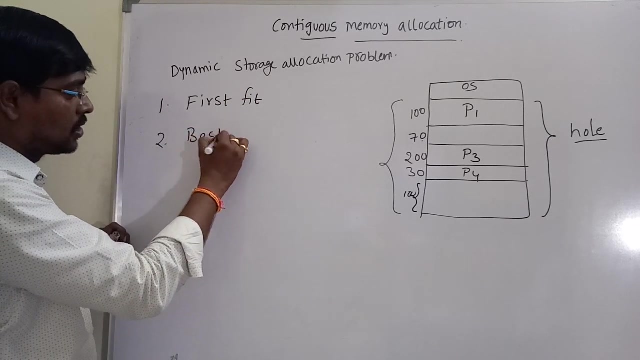 Suppose I am requesting a memory of size m, m bytes. Suppose I am requesting a memory of size n, How you will satisfy your request. So for this dynamic storage allocation, we have three test strategies. One is first to fit, best to fit, worst to fit. 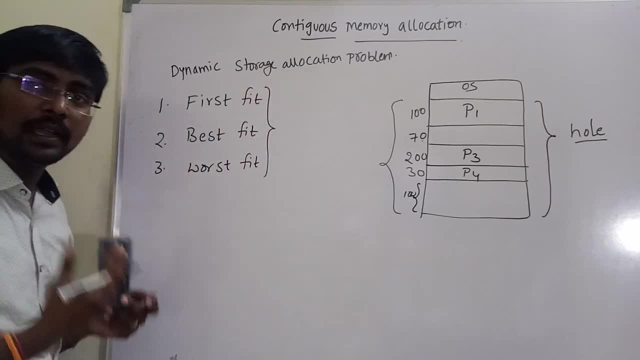 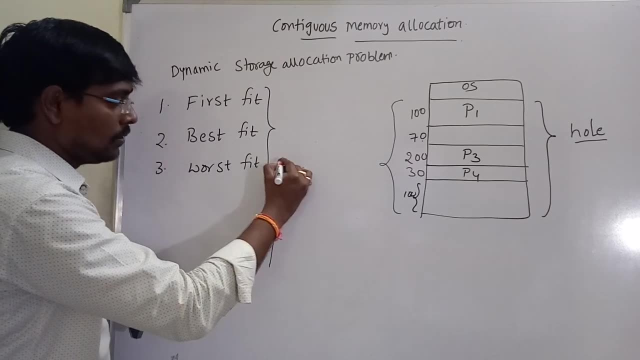 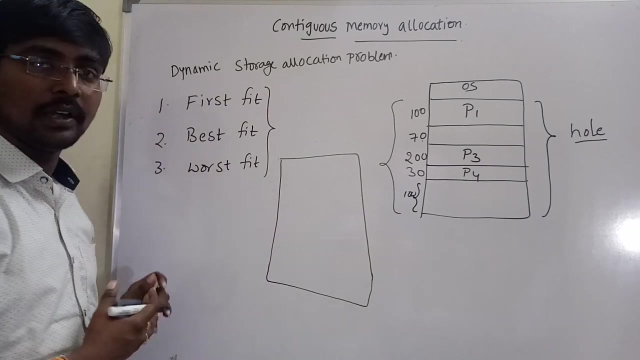 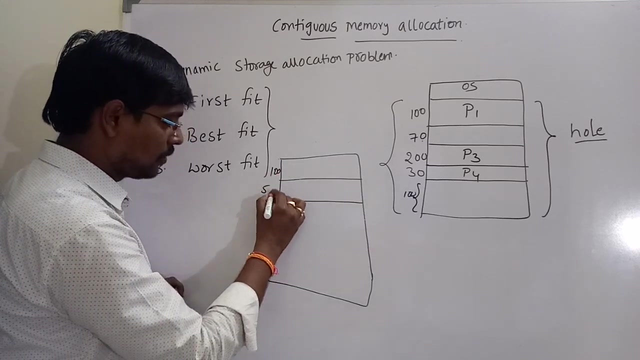 By using these three ways, we are dynamically allocating the process of our request. For example, this is the memory. After some insertions or deletions, the memory is divided of different sizes. Assume this is some 100, 50, some 200, 150. 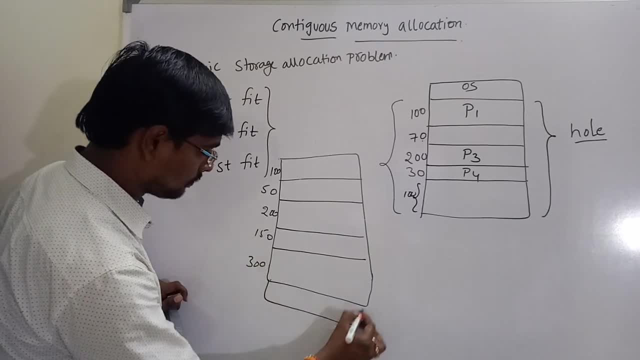 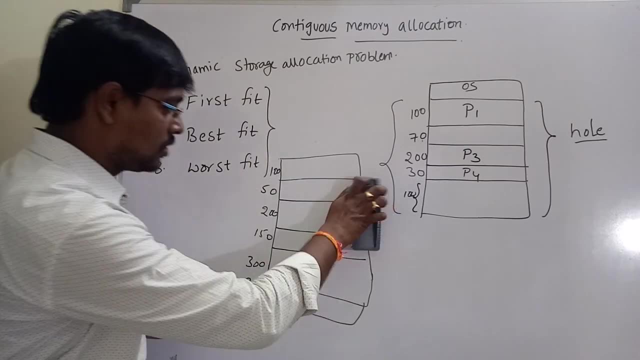 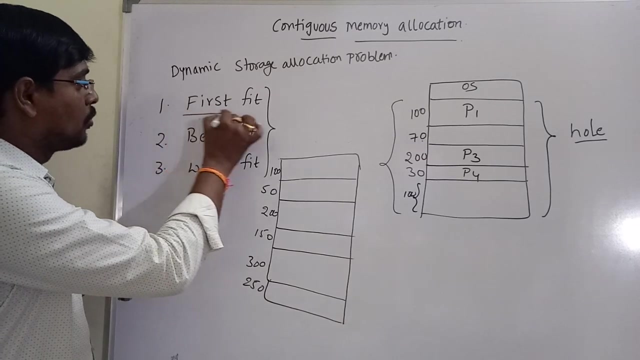 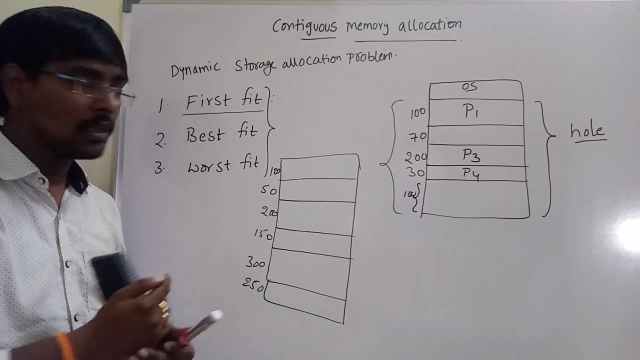 Suppose 300, 250.. These are sizes of each block. Assume these are the sizes of each block First to follow. the first to fit approach. What is the first to fit approach Whenever a process request for the memory in the first to fit? we are searching from the starting. 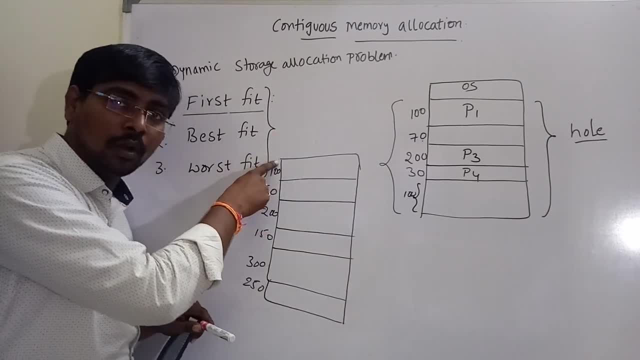 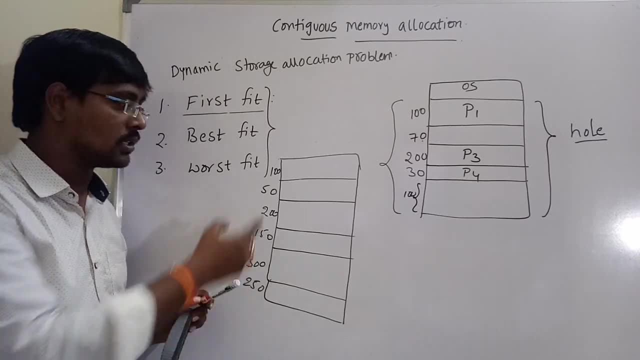 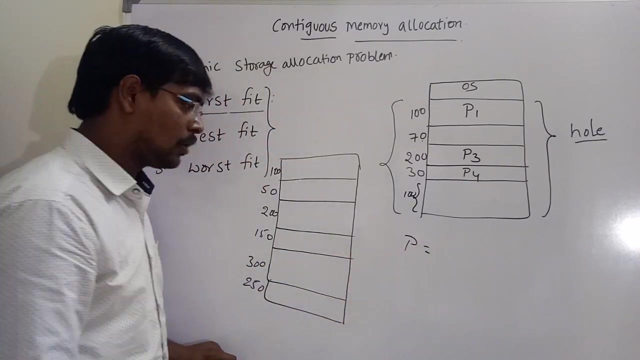 Assume we are searching from the first to free hole, If a first to free hole is sufficient for that particular process, If the hole is sufficient for the process we are allocating- Suppose my request, suppose a process of size 150.. How we are allocating the memory. 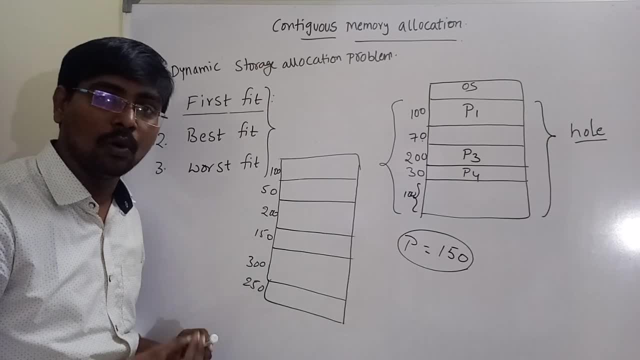 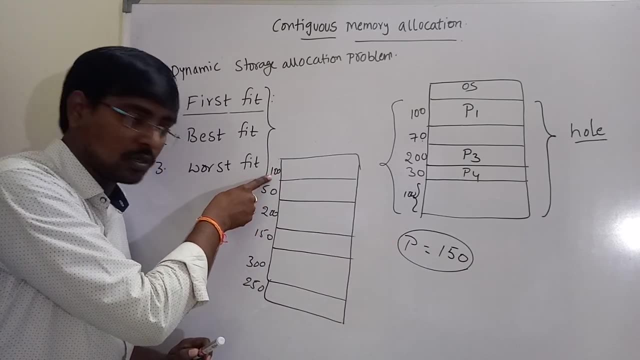 In the first to fit approach, we are checking for a free hole that is big enough to store the process. First to P is taken. This size is 100. It is not sortable. This size is 50. It is not sortable. 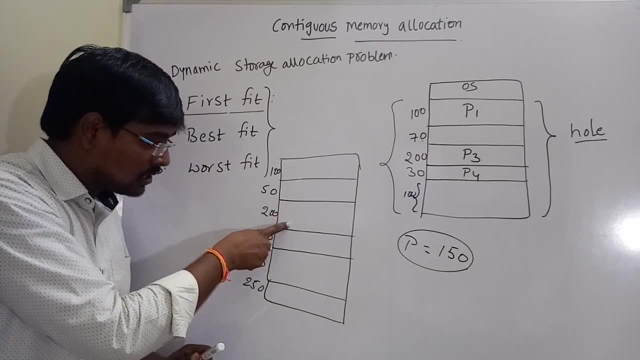 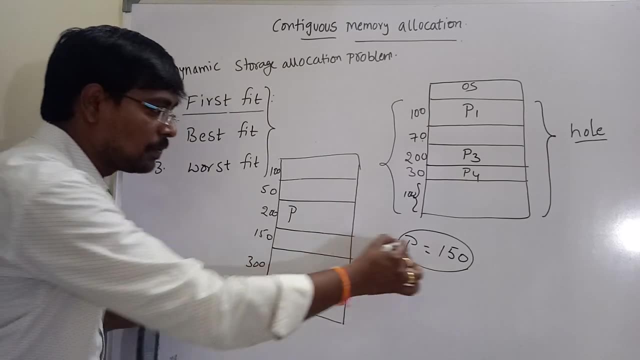 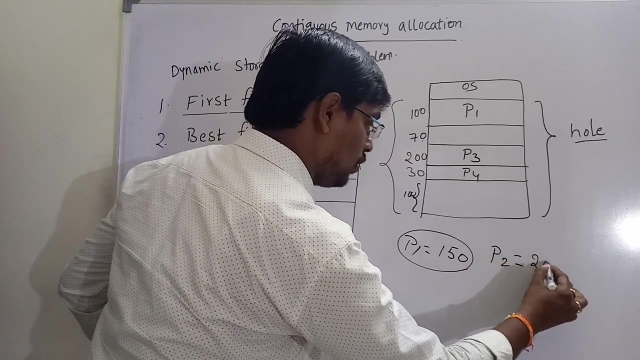 What is the size of this process? Here the block memory size is 200.. Our 150 is stored in this position, So P is stored. Suppose the P1.. P1 is stored at this position, Assume P2.. Suppose size of P2 is some 200. 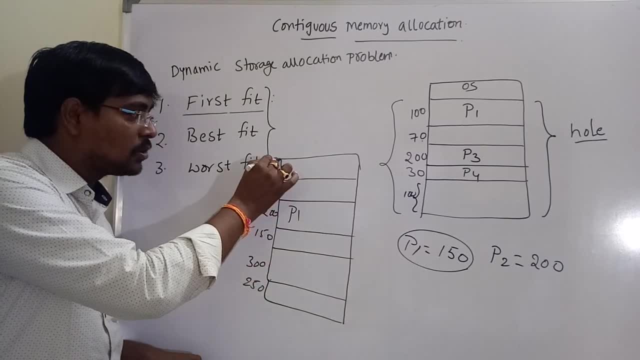 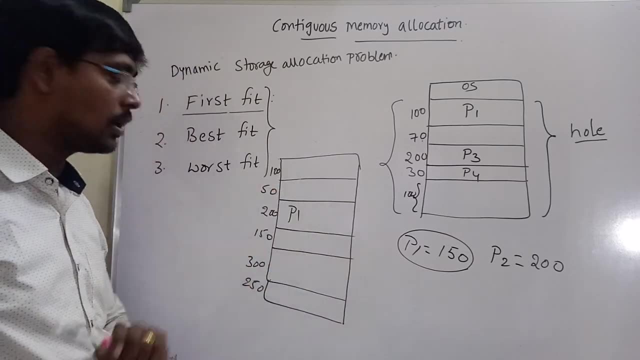 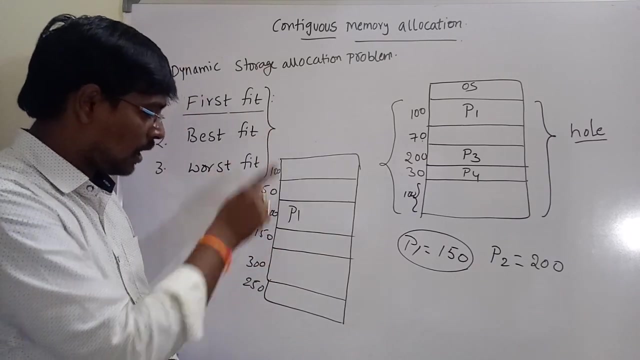 Size of P2 is 200.. N is set from starting Position. Or we have one more way. Always we search for the required memory from the starting position or search from previously stored position. That is, we have to search from this position or from this position. 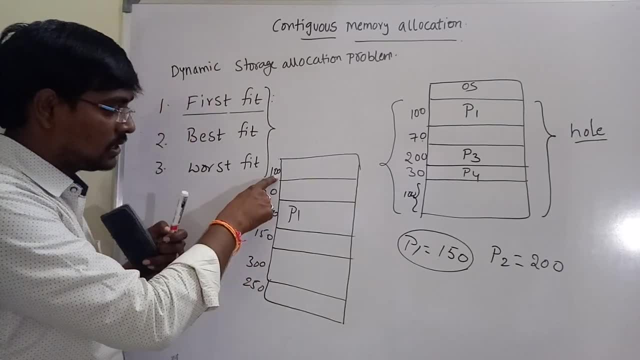 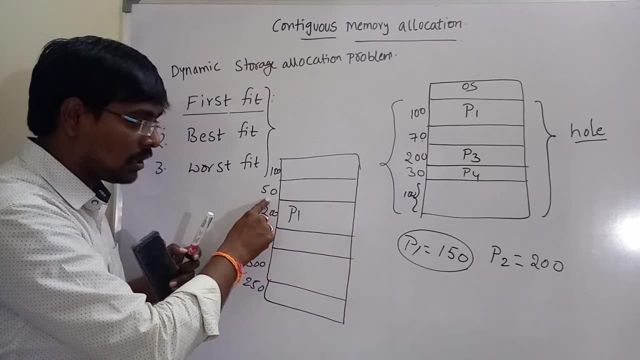 Suppose I am searching from starting position, The size is 100.. It is not sufficient. The free size is 50.. These are the free sizes. The free size is 50.. Not sufficient Here, the size is 200.. But the 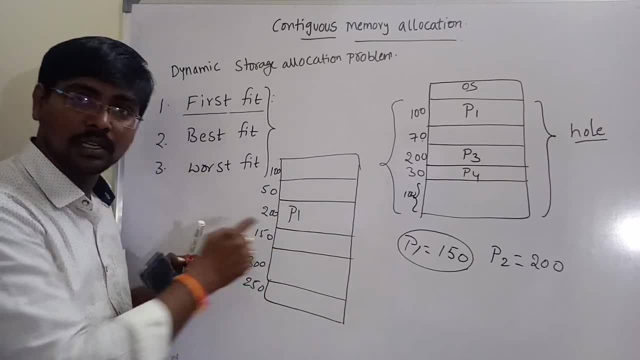 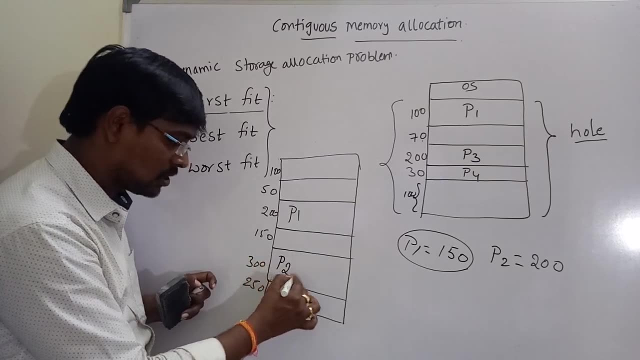 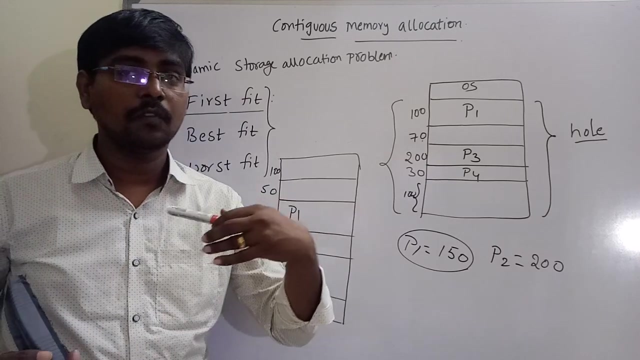 It is already allocated, Even though the size is waste. It is already allocated 150.. Not sufficient: 300.. So we place process P2.. We place process P2.. This is the first fit approach, That is, we are searching where the first hole that is big enough to store the particular process. 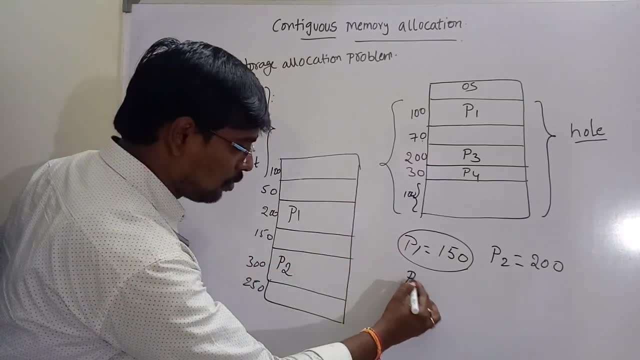 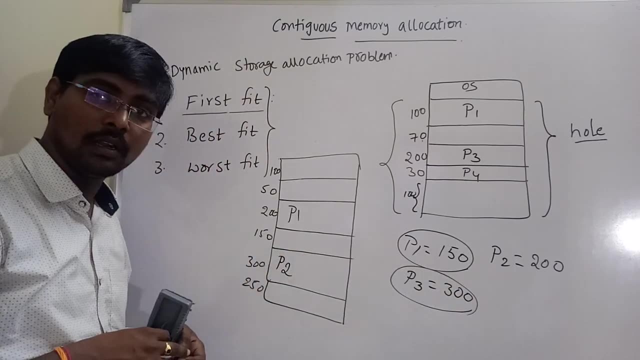 Observe By observing, Suppose, if you have one more process, P3, of size 300. Where we are storing 300. That is where we will store P3.. So the first fit approach is not suitable Move to best fit approach. 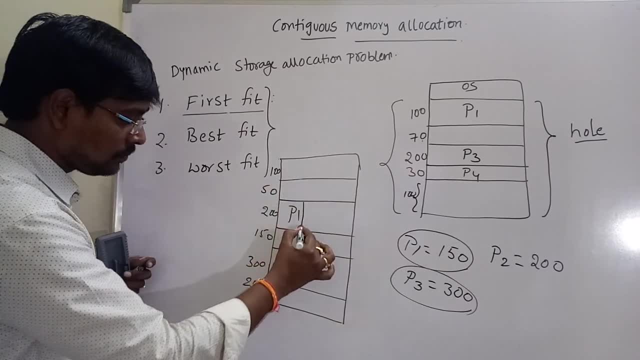 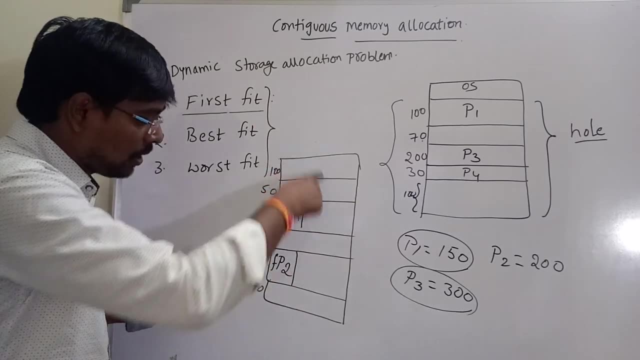 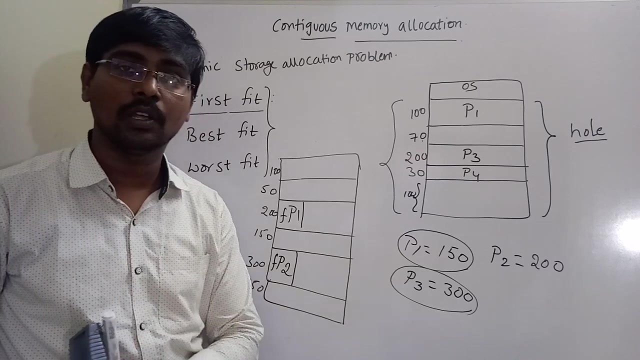 Move to best fit approach. Suppose This is first, This is first In the best fit approach. From the starting to ending we search The best fit approach. from the starting memory- free location to end, free location. We search Where it exactly fits. 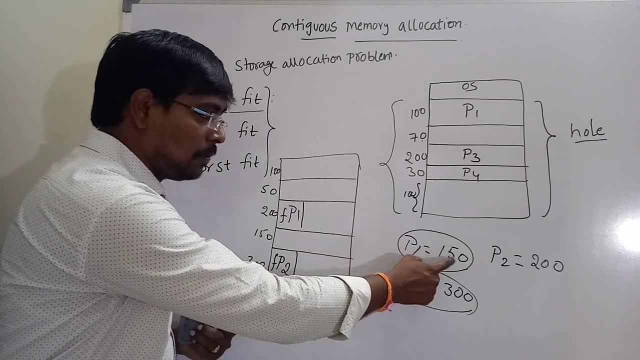 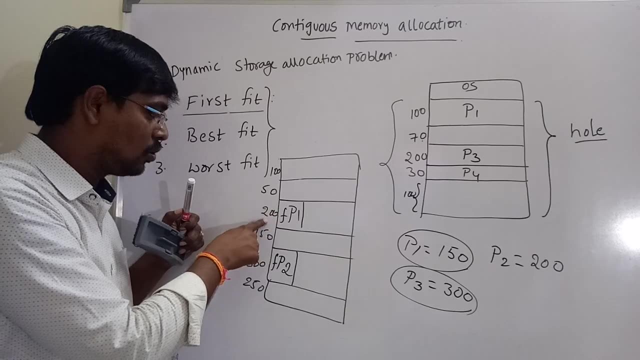 That is the lowest possible requirement. For example, First process, 150.. The size is 100.. Not sufficient 50.. Not sufficient 200.. Even though it is sufficient. Scan the entire memory. So 150 and 150.. 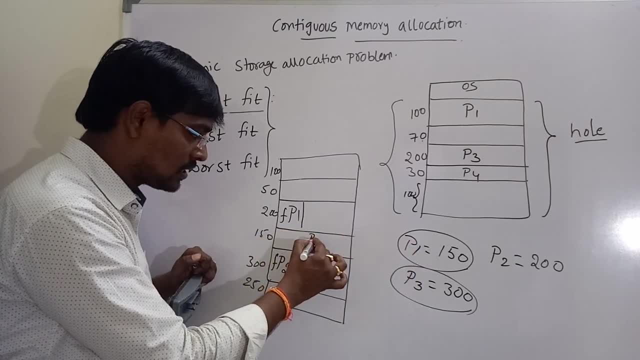 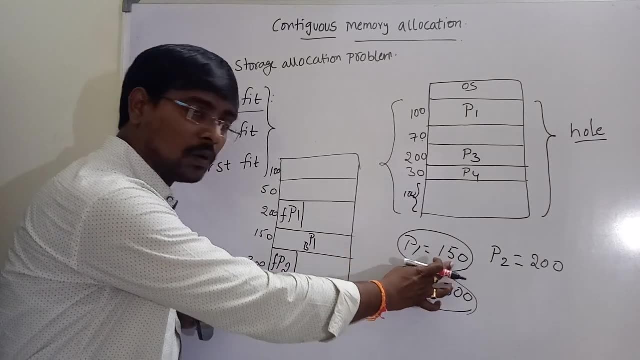 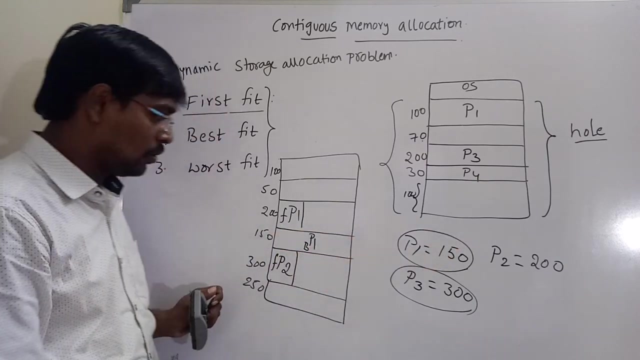 Exactly same. So process P1 is allocated In the best fit. Process P1 is allocated. Suppose Process size is 140. Nearest to 140 is 150.. So 150 is allocated Next to process P2.. 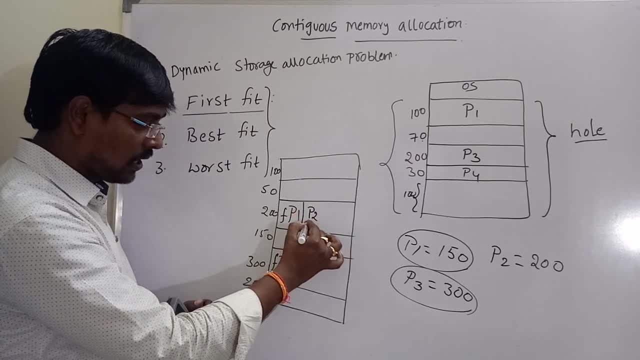 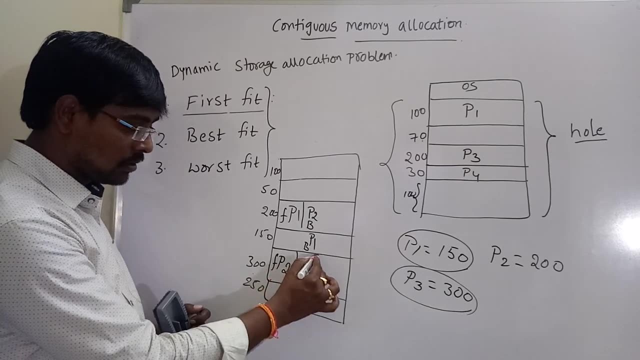 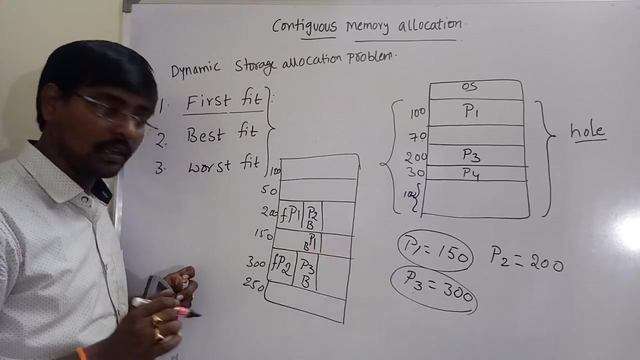 So again start from the set Process. P2 is allocated. in best fit Process P3 also have same space. See this one In the first fit. In the first fit Process P3 is not allocated, But by using best fit. 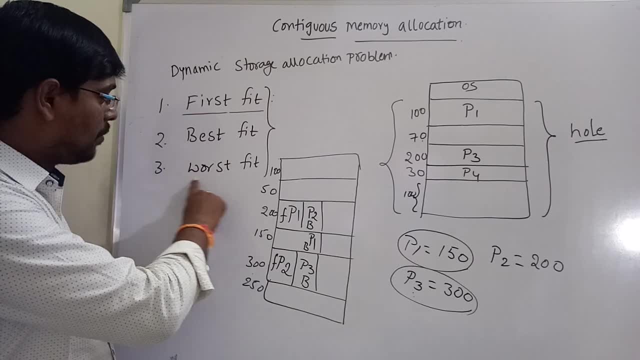 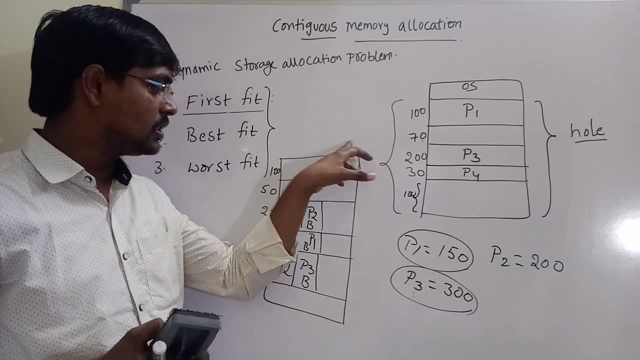 Process P3 is allocated. So we start from the set Process. P3 is allocated, Ok, And move to the worst fit. Worst fit means similar to best fit, Exactly reverse In best fit. we search the entire free memory locations. 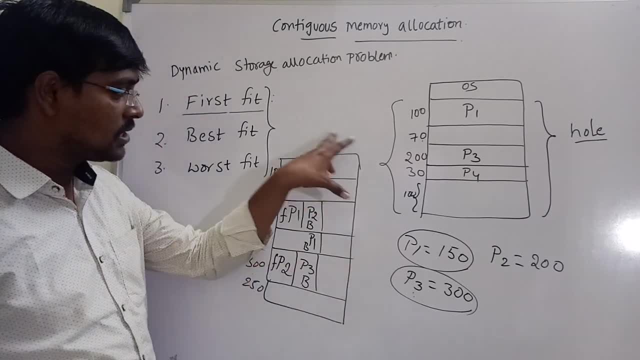 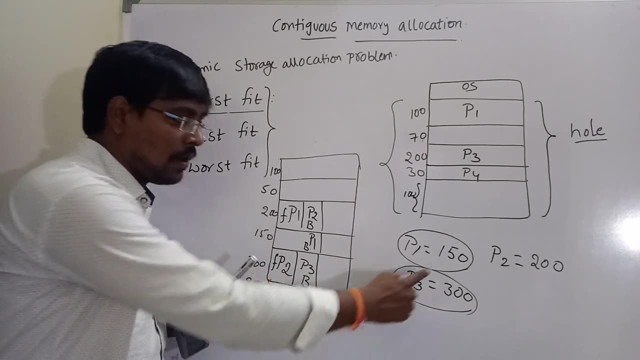 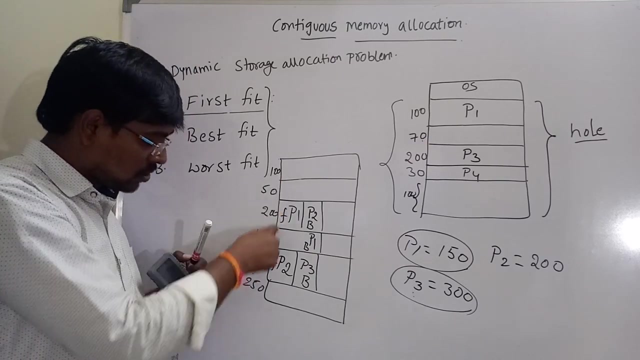 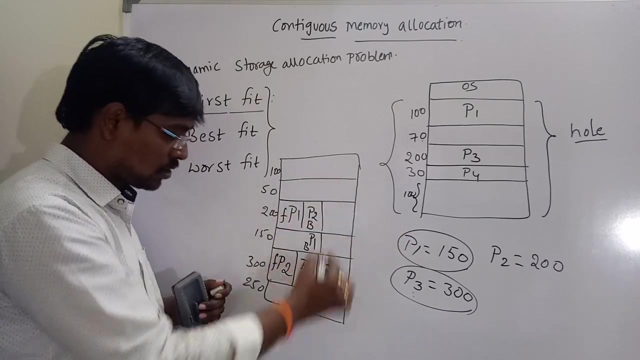 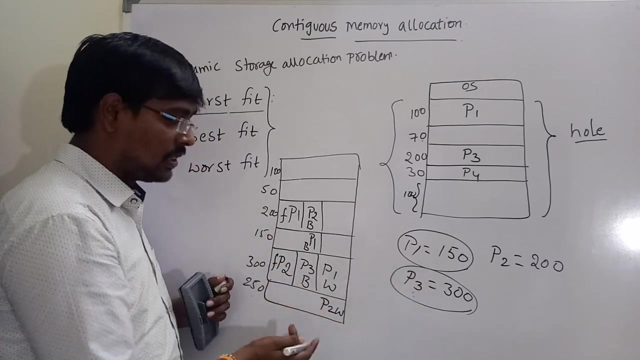 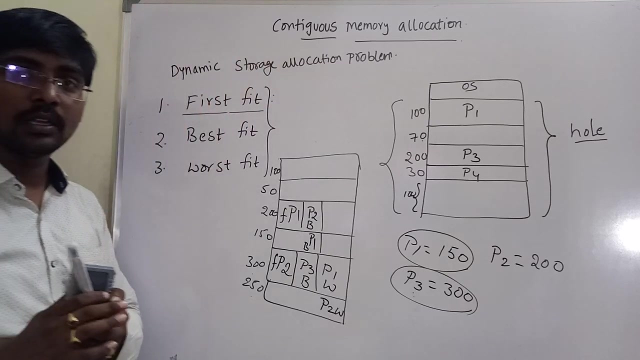 That is best suitable is allocated In this search entire location. That is the last suitable, That is the worst suitable location, For example, 150.. First, process 1 is allocated to the largest pool. So what is the largest hole? 300.. So process P1 is allocated at this position, Process P2.. Next one is P2.. Size is 250.. This is the first position. Next, P3.. There is no variable space. This is the way to allocate the memory. This is the problem of dynamic storage allocation. 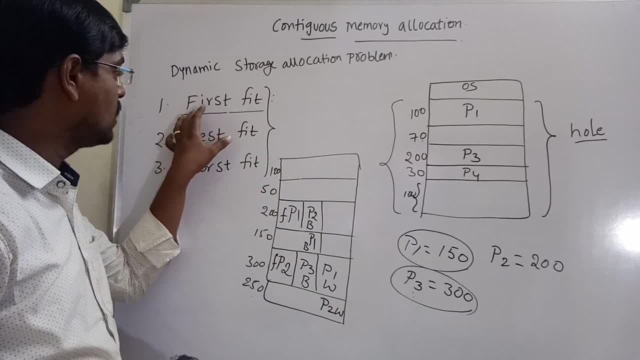 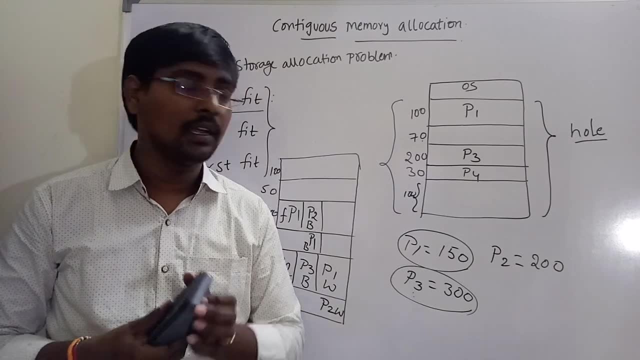 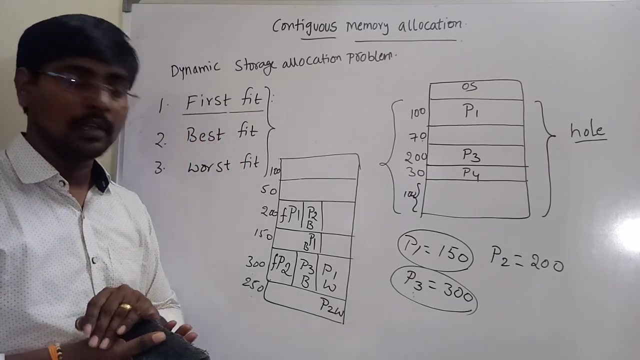 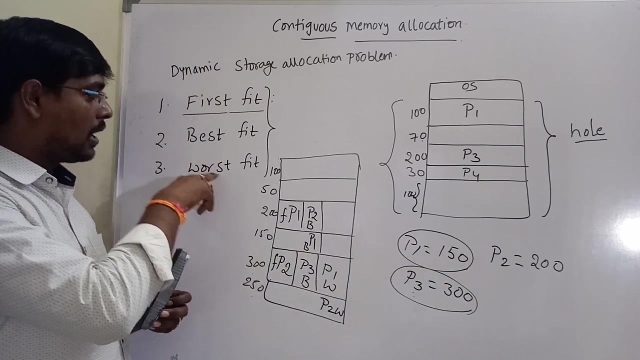 This dynamic storage allocation problem is solved by using any of these things. Remember: best to fit, first to fit, worst to fit- All those are. there is no guarantee that which one is best, Depending on situations. in one situation, first to fit is better than best to fit. You think that in this situation, best to fit is better. But depending on the situation, first to fit is better than best to fit And worst to fit is always a maximum waste case. 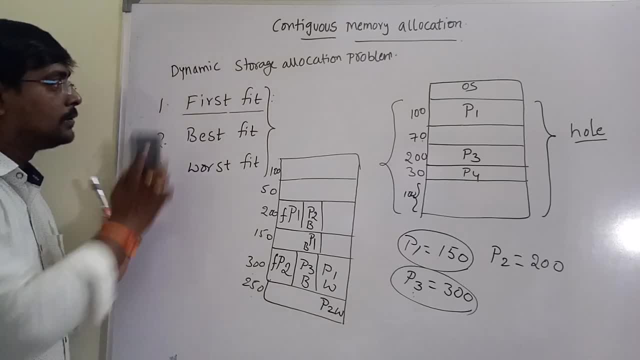 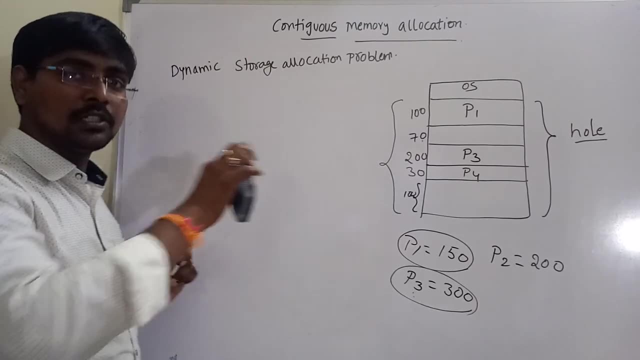 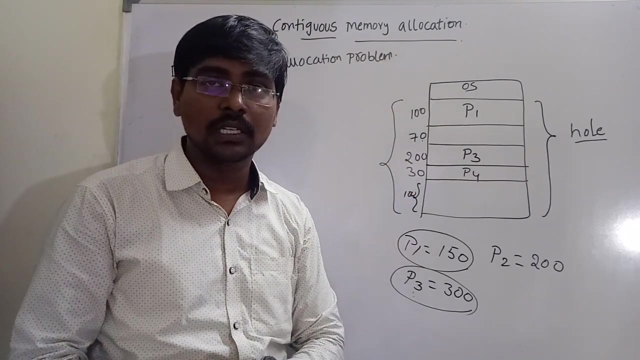 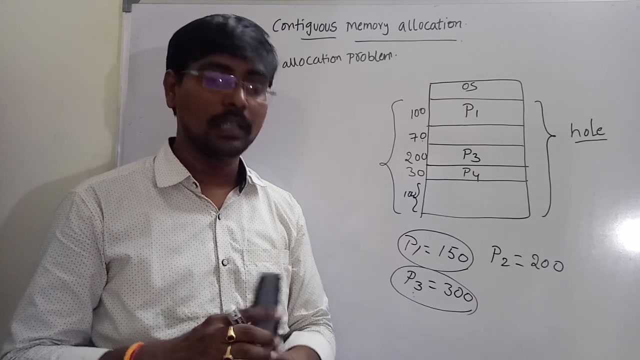 Okay, Dynamic storage allocation problem. Problem End: Okay, It is clear And move to previous one. So what we will discuss In the fixed sized partition or variable sized partition. Suppose the partition size is 100 bytes. Partition size is 100 bytes. If my process size is only 70 bytes, What about remaining 30 bytes? What about remaining 30 bytes? That is called fragmentation. 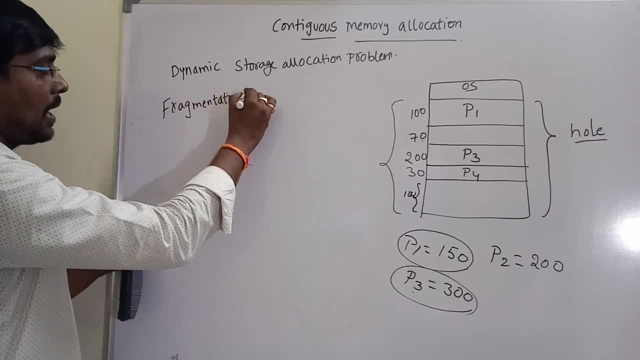 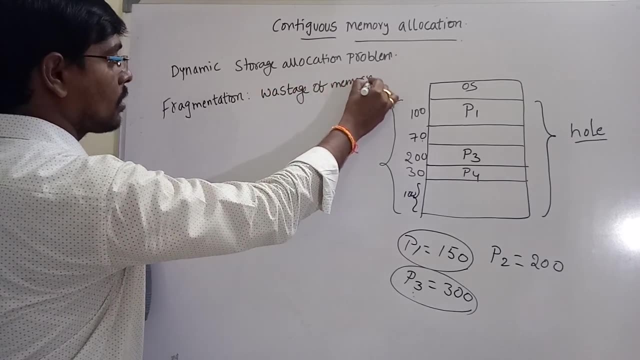 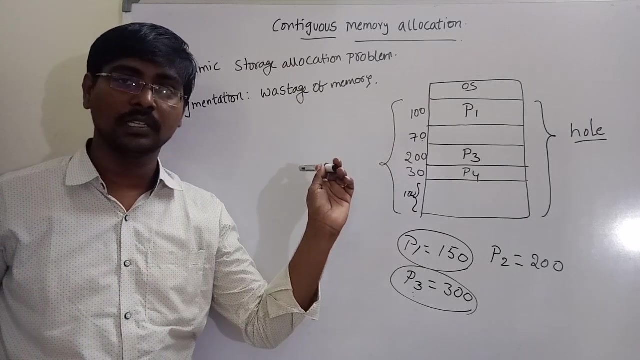 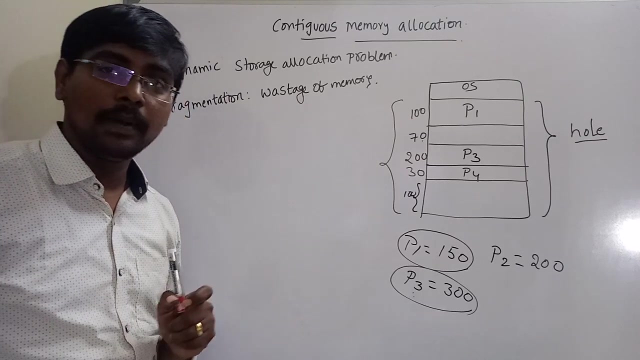 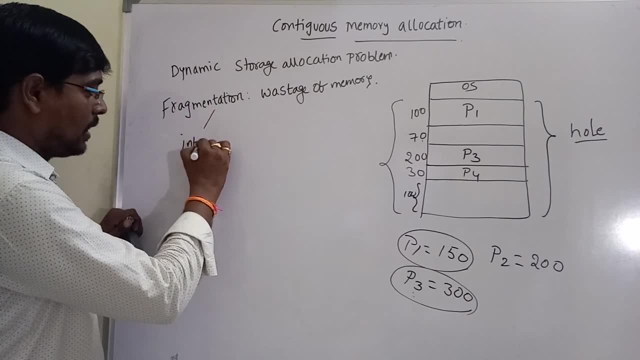 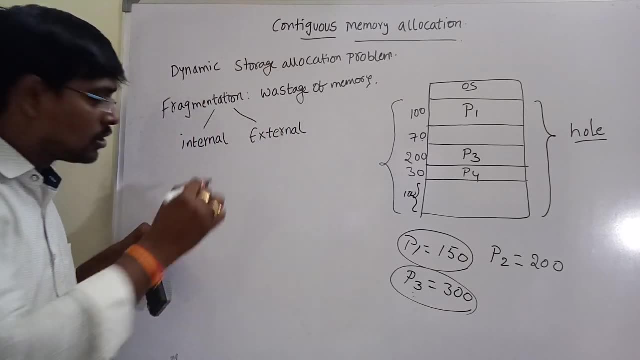 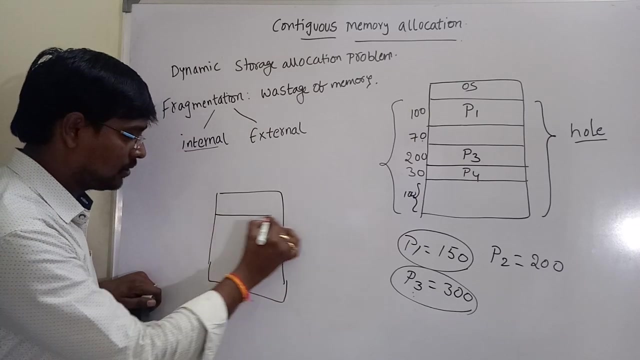 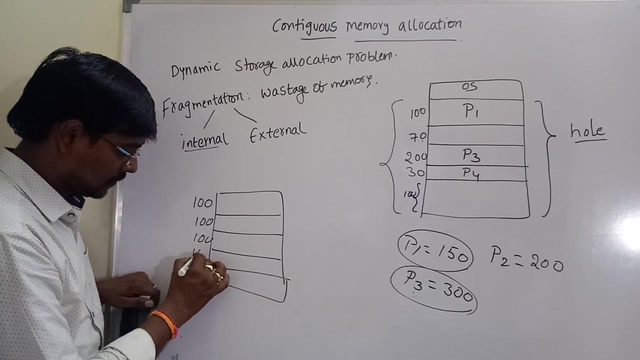 We have two types of fragmentations. One is internal fragmentation. Second one is internal fragmentation to one is external fragmentation. so we know internal fragmentation. internal fragmentation is this one. this is the internal fragmentation. suppose the size is hundred. the size is hundred hundred divided into fixed set of partition. 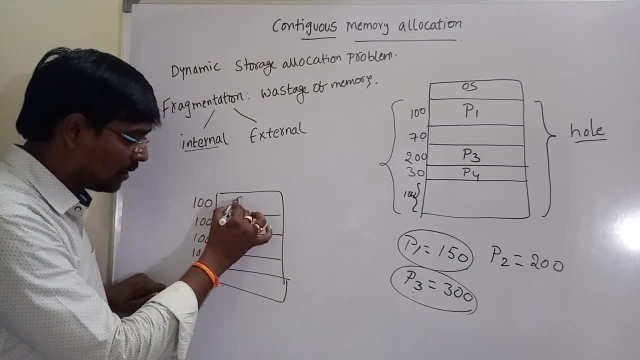 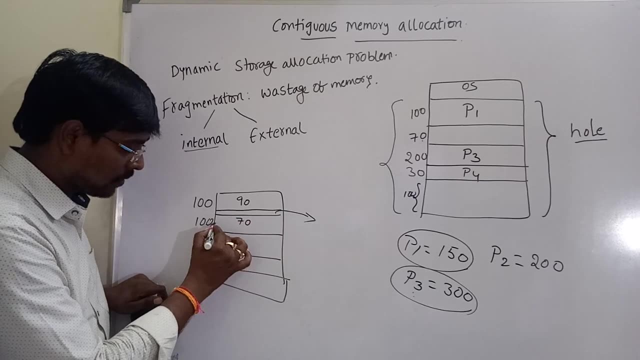 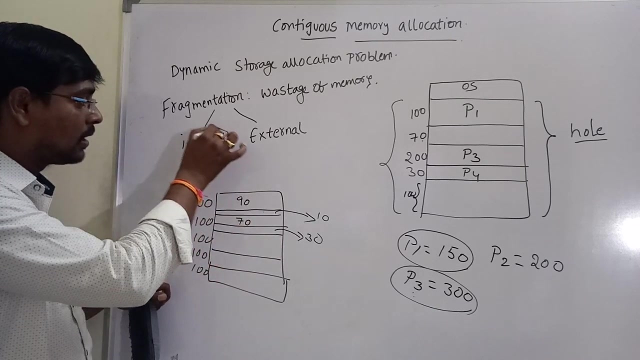 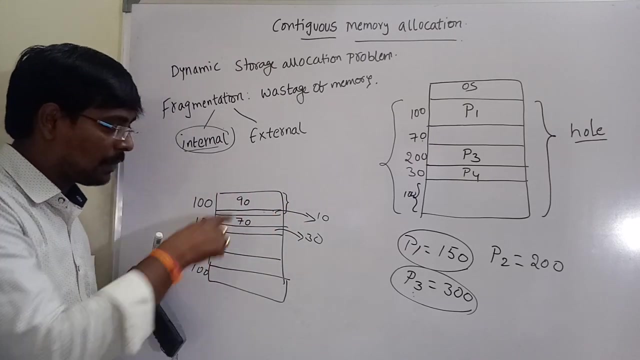 suppose I am allocating a process each of memory 90. what about this remaining 10 bytes? suppose I get a process of 70. remaining 30 bytes, remaining 10 bytes. so it is waste. internal, internal means. we are allocating the memory to this partition. I am allocating the memory, I am getting this partition, but it waste. 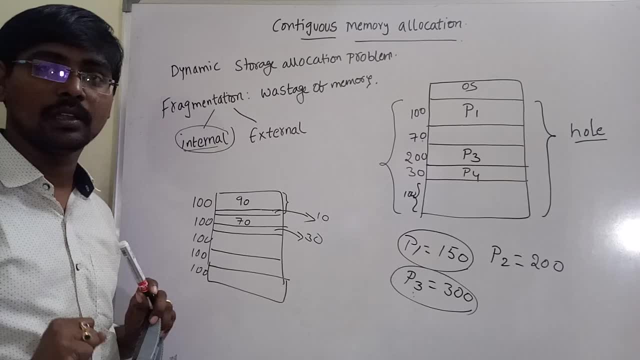 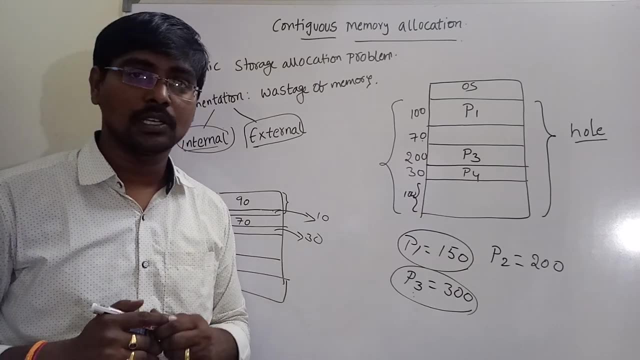 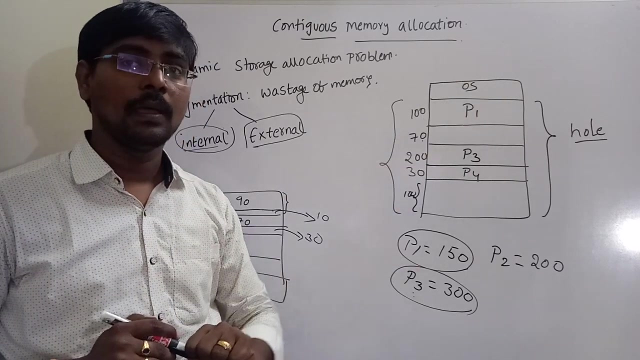 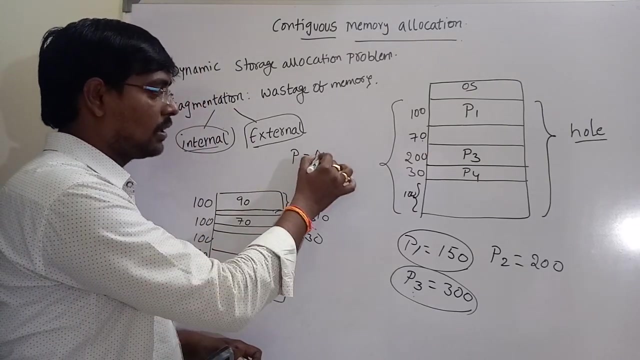 10 bytes of memory. this is called internal fragmentation. but move to external fragmentation. this is the important part one. what is external fragmentation? suppose the available memory, suppose the required memory is available, but it is not contiguous. it is not contiguous. for example, I have a process of size hundred. what we will do. so hundred is available.